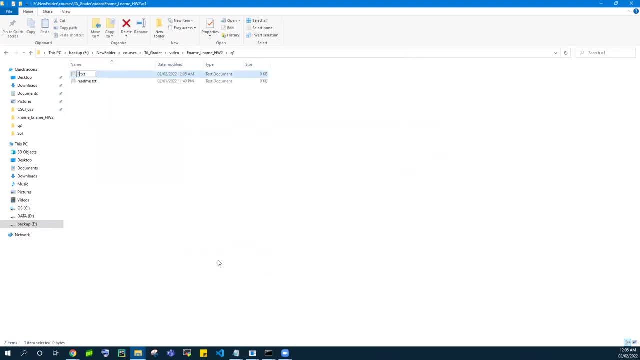 and also have another listener for it. So you could have, say, question one listener and you're going to have one list file. select question one editor. obviously you know if it's one A or question one one or one A. however you want to name it, just name it accordingly, but just make it pretty intuitive. 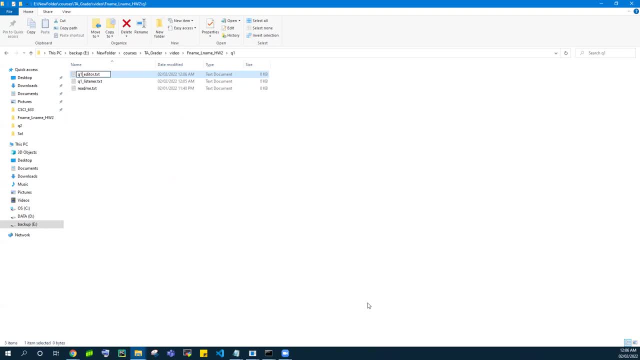 We don't want to rack our brains about what exactly. which question are we referring to, and just change the extension list. So now we have this. This is something that we're expecting. Now, when you open this, you're going to get an empty list thing. 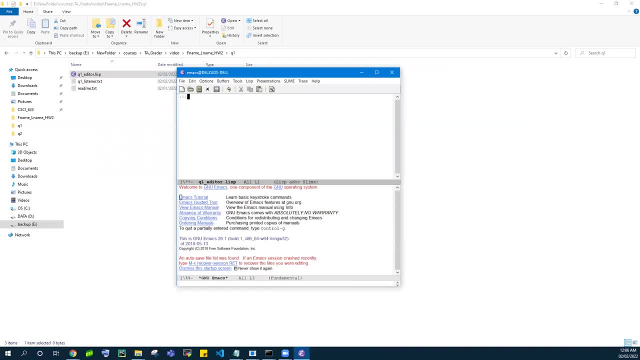 I want to take you on over comments. So this is a comment. any, any semi-colon is a comment. but, like, if you've used markup languages you might know we have different levels, like, say, for HTML. there's like there: 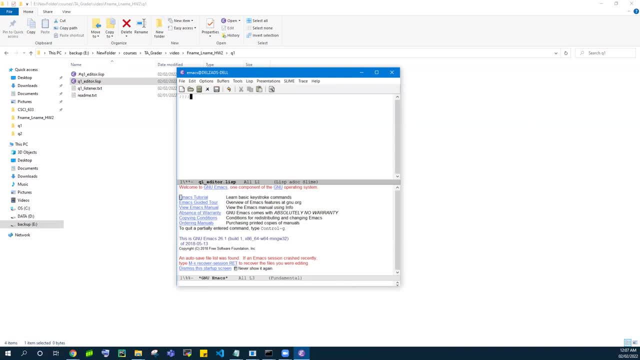 is an H1, there's an H2 tag. Similarly, here we have like a basic comment has four semi-colons. then you can keep increasing or decreasing them depending on the level of your comment. Now, initially, let's say you want to say something about what the function does, or 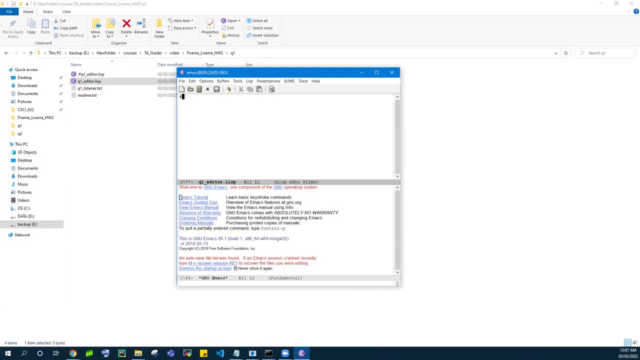 you've created a function and you want multi-line comments, so you might have a hash line nine, nine, Okay, and have just write whatever. so this function does blah, blah, blah and that's how you can write. now one very important thing i want you all to know about: uh, your. 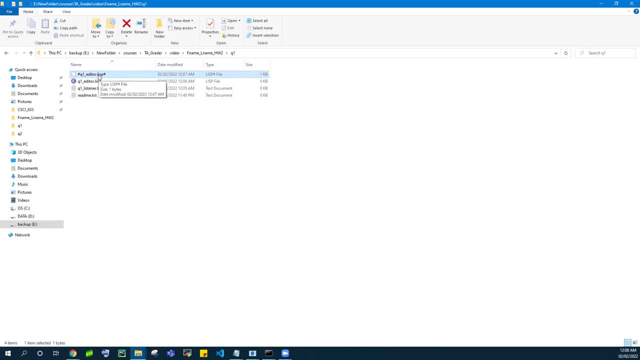 yeah, you don't need to submit this, uh uh, this compiled file, because it's not very useful for us. but if you submit it, it's not going to be a big deal. it can exist. um, just make sure that it it's. it has these codes, it has these hashes around it, because that will let us know, and also this extension type. 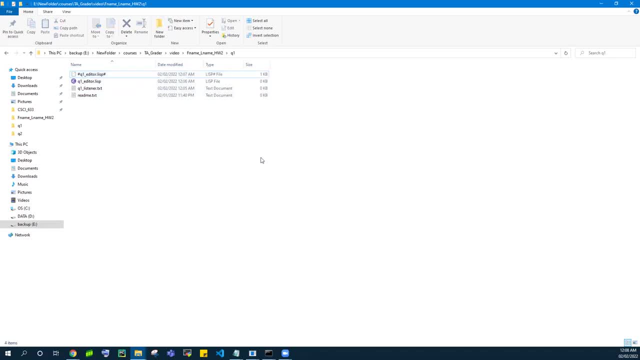 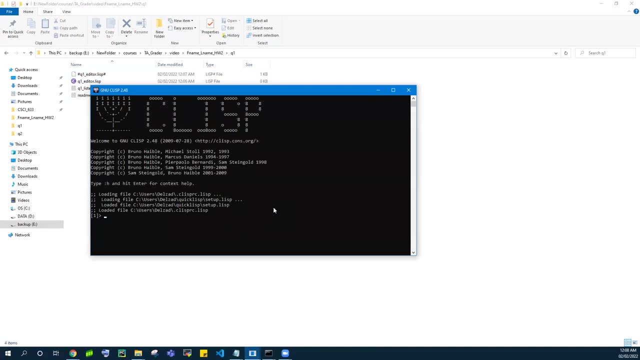 that is the compiled file. it's not your list file. yeah, so, coming back to if, if, if you're running something in list, remember to add these brackets. these brackets have a meaning behind them. a lot of students have made this mistake where, unnecessarily, they cross marks, where they do something like this: 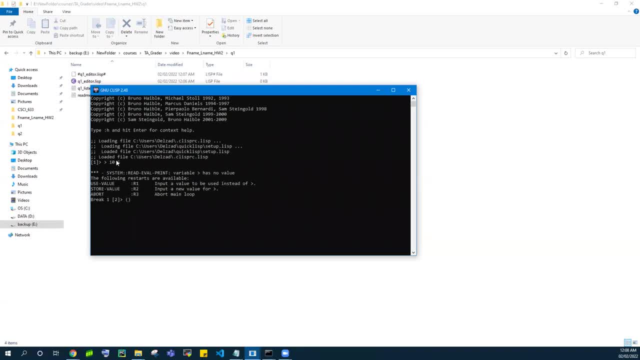 this is what you're going to return if you do something like this, but the exact same thing. brackets get some value. this has no meaning in this. maybe it could be a specific editor that you guys are using, but if it was that case, then it would have been nice. 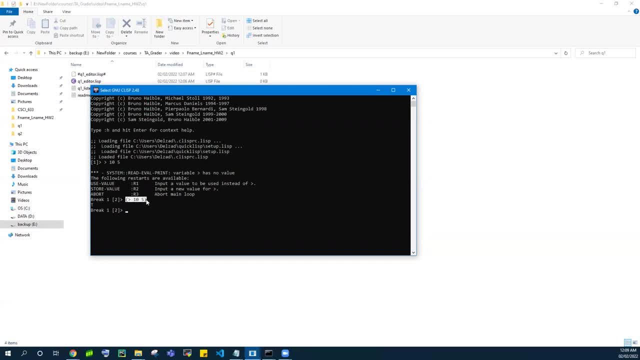 to know, uh, but in general, lisp by default uses brackets around it. uh, and that is uh, that is something that is mandated by this or that's how it works. so, say, this is what you ran and we in this question we weren't looking for errors per se, so this is my output, so i'm going to pull. 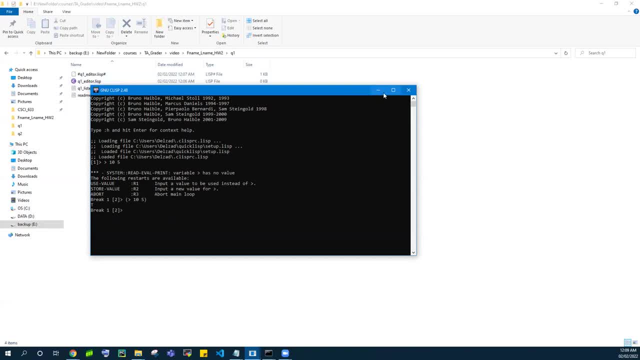 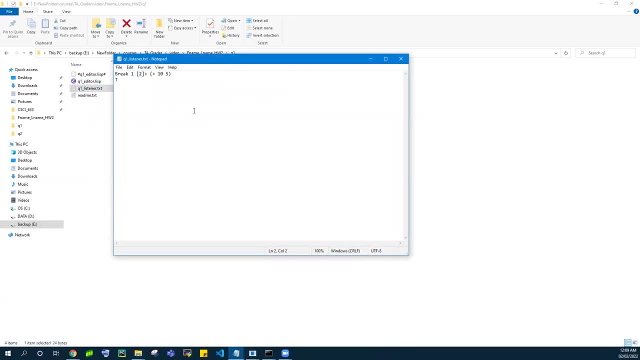 everything from here to here and i'm going to put it in my listener. and now this is my listener file, as simple as it can get your command and the output that your command produces. now, say, you're using a function like, say, for my question two, let's take a look at your uh program that you did for homework. one, 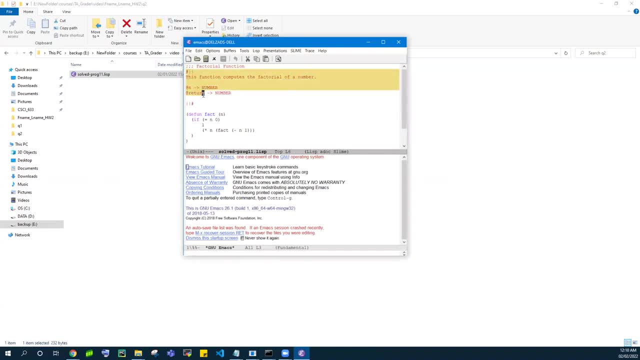 you have this, so you have add in these comments multi-line comments. uh, i just added these to be fancy. you don't need to, but this is how usually comments are written, where you write the input type and what is getting returned. so, uh, yeah, so we talk about all your functions and everything. so when you're reading a function, 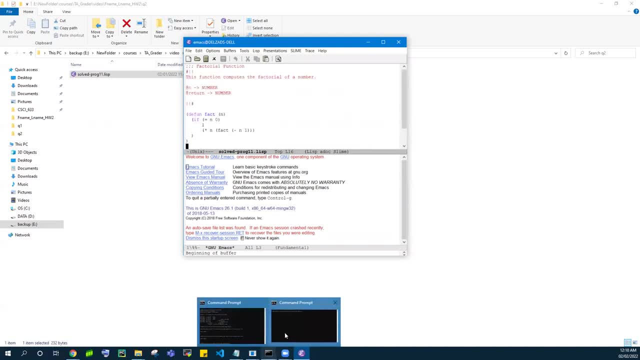 if you, if you want to run it on the command line itself, then you're going to want to have to add a print statement so that it can print directly with the function name. uh, don't worry about read too much, it's, it just takes uh command line arguments but 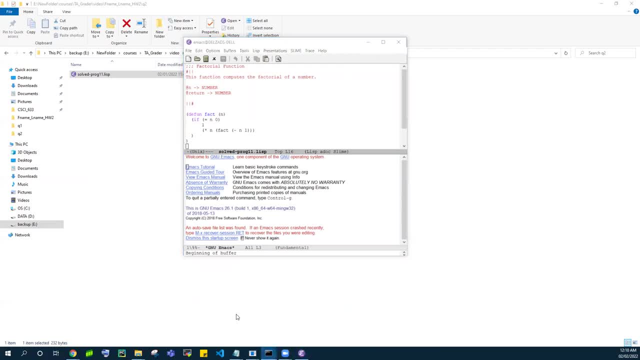 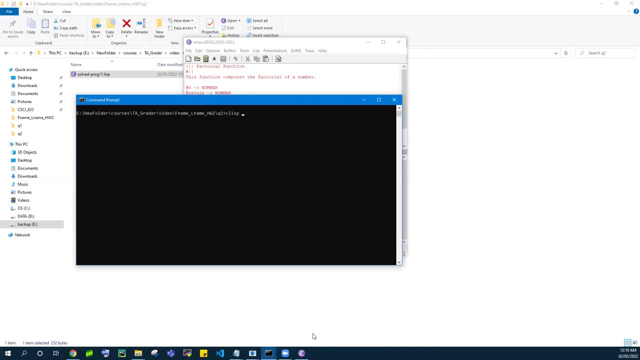 that wasn't a part of your uh code, that was a part of your homework, so don't don't take too much stress about it. say, i try this. it's gonna ask me for a number to take this, so this is what my output comes to be. so, since i'm doing this on the command line, 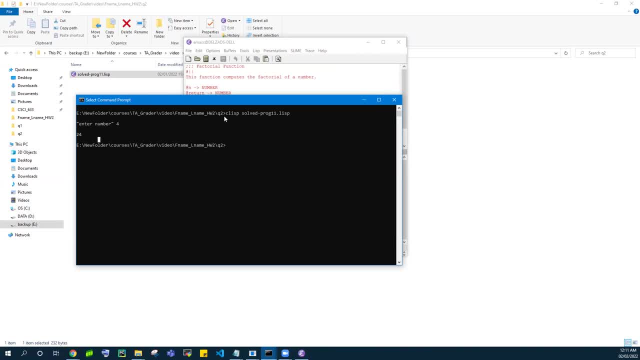 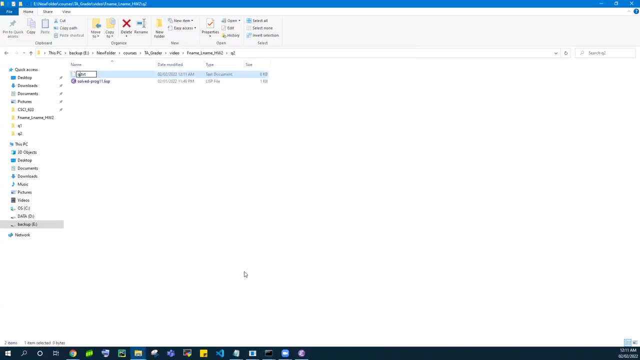 i would take this. you don't have to take your paths. i don't want to know where you saved it, but this is what's important. but you might just want to be like: take the entire thing, you paste it in your listener listener and space it here if you don't want to share this, just be like. 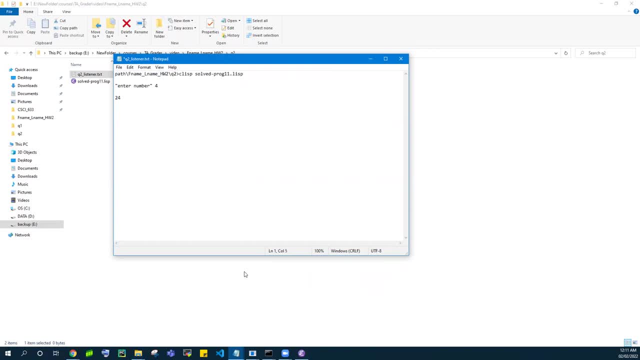 maybe all the way to here and just be like paths. we don't really care, but as long as you, we see the command that you've used, uh, your uh output also is important and whatever other stuff that the command usually wants to show. uh, let me talk about 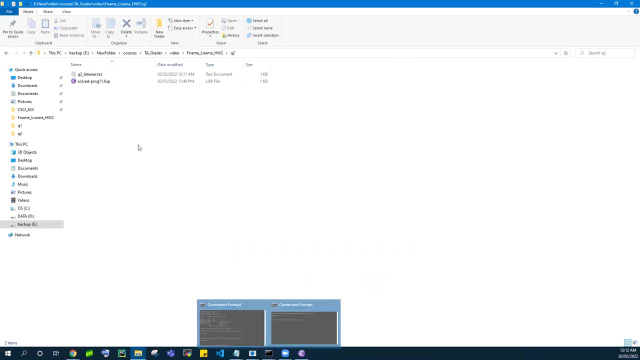 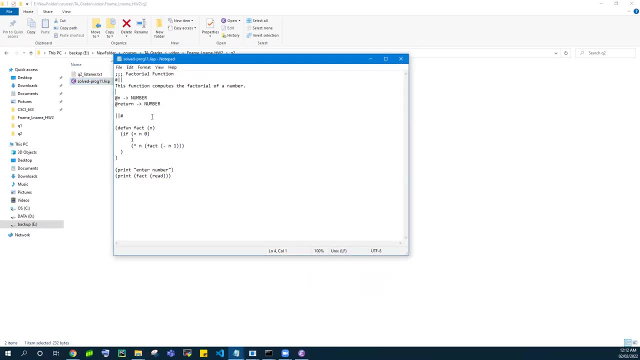 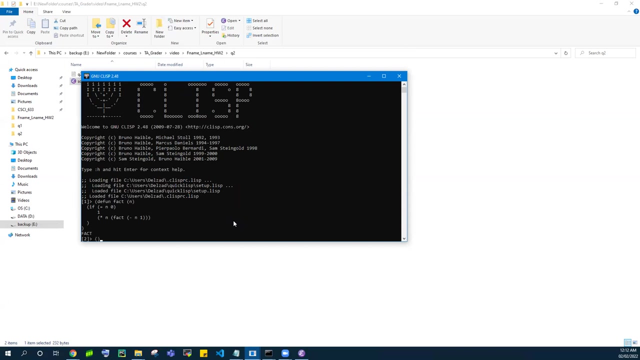 race a lot about race more because, uh, let's say, i think this gram, let me copy everything from it. actually, i just need this, so if i have a function, i can trace that function so that both of us, the students and, uh, the graders- everybody can understand what's going on behind the scenes. 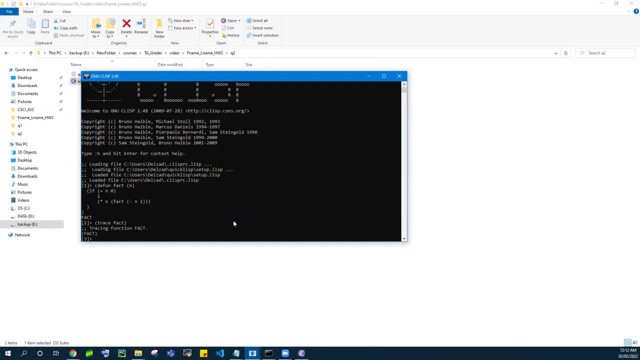 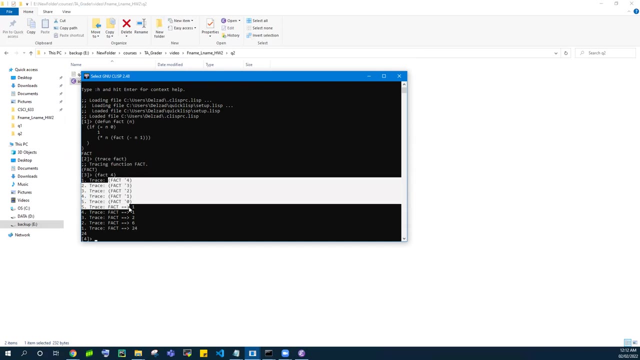 uh. it'll be very helpful for y'all also to understand how things are working. there we go. so after you run your code with a trace enabled, it's going to tell us each line of uh implementation. so it'll go like four, three, two, one, zero. it goes all the way to zero and 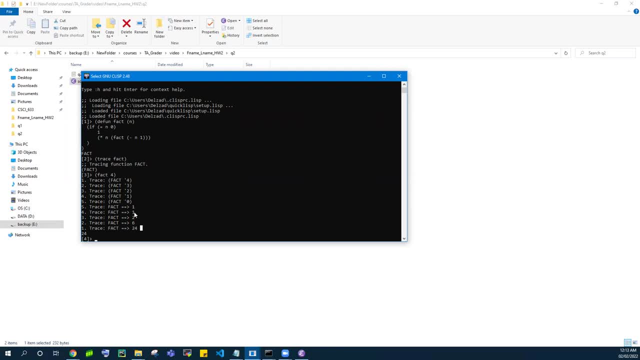 hey, where's the zero supposed to return? return what? so? leave one, one, two, six, four and then you get your twenty-four. now, if you want to stop tracing a specific uh program, you can just uh, be like untrayed and move. it's unfocused. you could trace multiple uh programs at the same time. so say, supposing you, 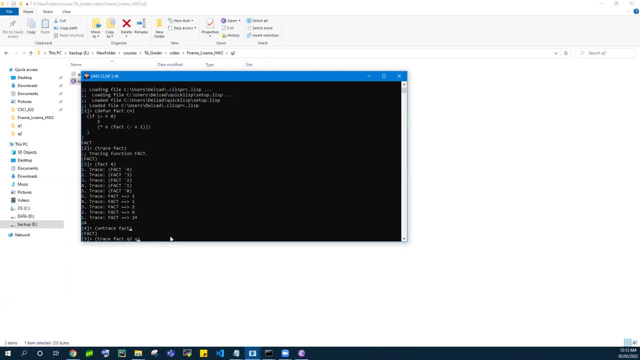 have one is fact. maybe you have something. question two, you have question three. you can just trace as many as you want and then individually call back up the whole list. that's so sort of great. and the last is to be able to, if you're asked to multiply, you lower the vueliciones. into so that you can put upper case. if you seek the second everywhere, then you can knowledge process. if you without um, you can just set vertical believe it to twice and anyway the opportunity. if i only mess up picture in my tengan, even though 고 weren't to narrow, it's gonna get four on the left side. i need to control it like jobs or go to multiple points and 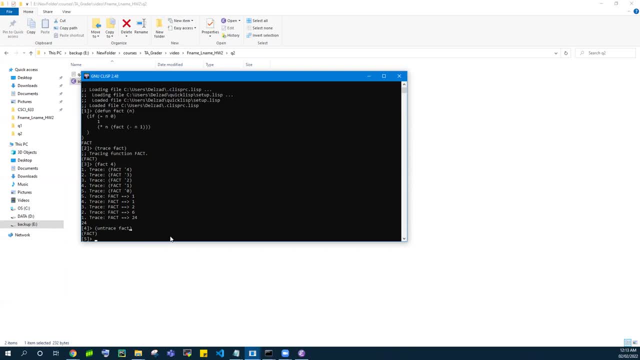 them So say you've traced all of these and then you can just individually say fact 4 and it will still trace it for you. Right now I have untraced it so it's not going to return a trace, but you can always remember that tracing will be helpful for you all in. 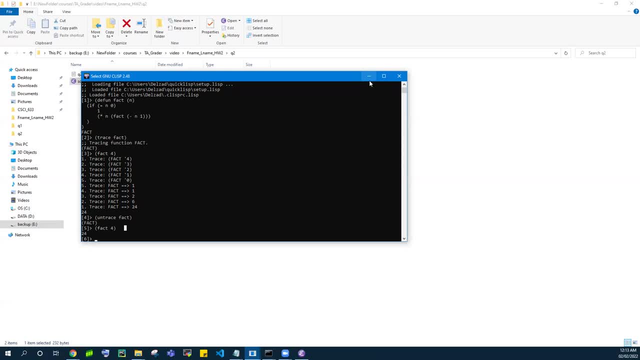 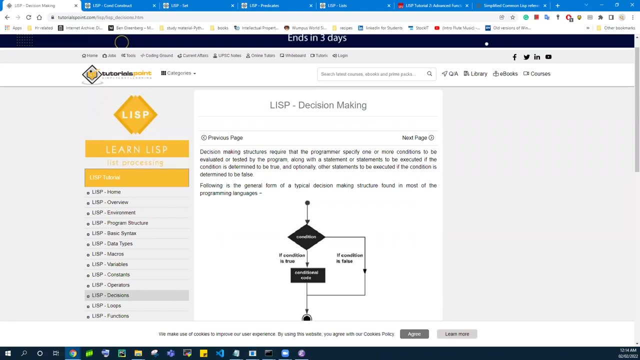 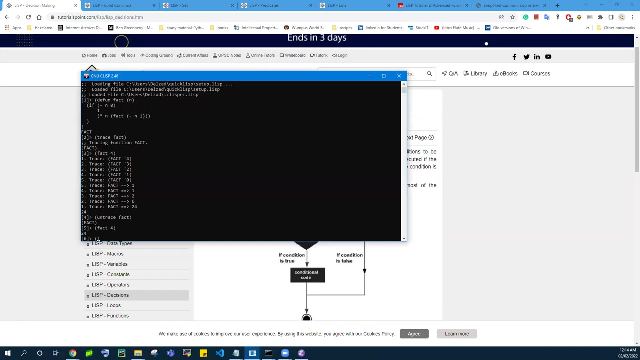 debugging. It's not required for all your programs, but why not? Okay, so let me talk about- yeah, let's talk about cons. So say at least by now, everybody should know what cons is. Cons is consecutive cell. It is a keyword in list which allows. 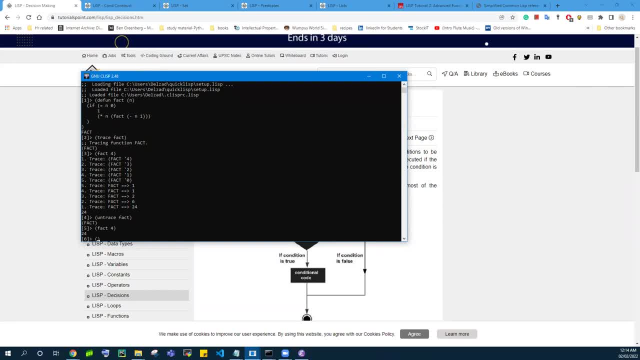 you to create a two-valued list, but you can always create a two-valued list. So you can always create a two-valued list, but you can always create a two-valued list. You can always nest them to create multiple lists. The first value is the CAR, the second 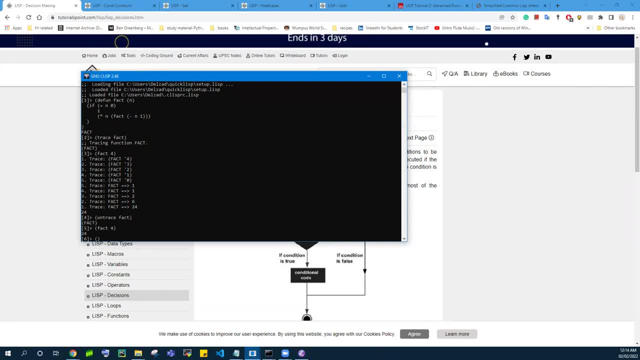 value is the CDR and your. if you select a CAR, your first value is returned. If you select CDR, everything from that value gets selected. So let me introduce. first let me introduce how to create variables. So def bab say, name is John, You have a name. 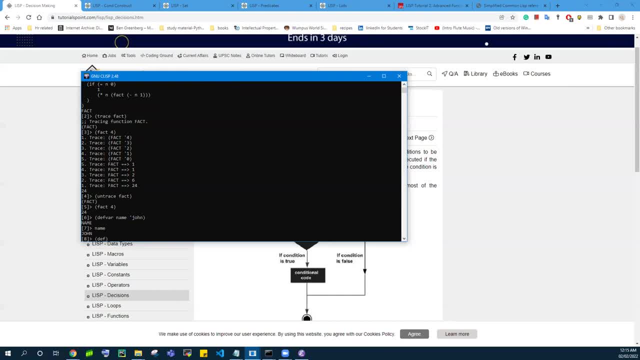 as John. Similarly, if you want to create, say, a list, then you're going to have to write def parameters For atoms or single-valued variables you might have. you can just use def bab. but if you want to create a list, a saved list, then you're going to have to. 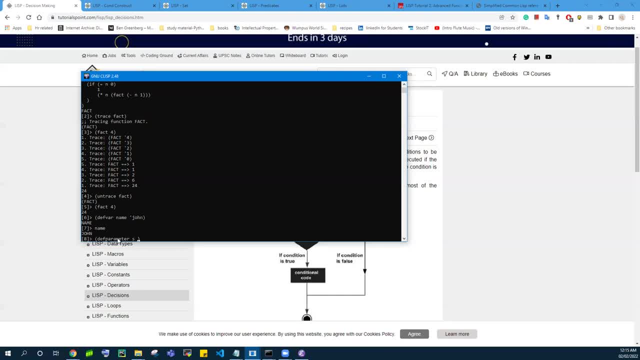 use def bab. So say, we have def bab S and we have a list of, say, cons and then we have cons A and B. You have S. S is going to give me AB If I want to nest my cons. 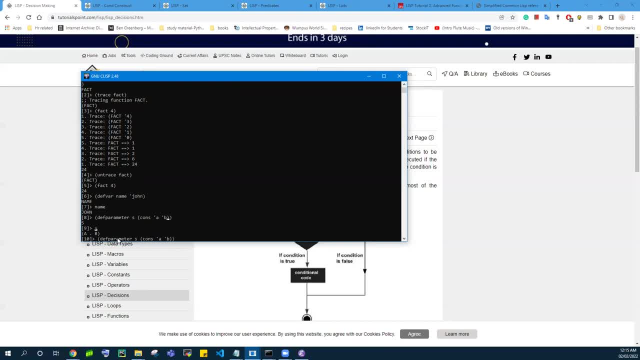 we already know how to do that, So let me take you through it again. Say: we have cons A. You're going to go inside, create. If you give me, add a bracket. you close a bracket A. cons B: 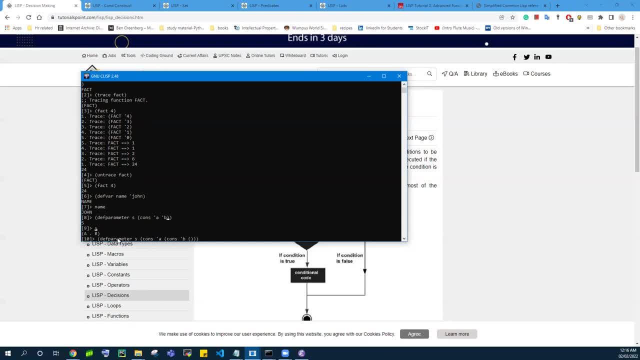 Add a bracket, close a bracket. C and nil. So in a list if you have C with nil, it's mostly the same. It just ends up because you're adding a cons to it. it's just going to become the same value. Nil is more like the ground if you're from the electronics. 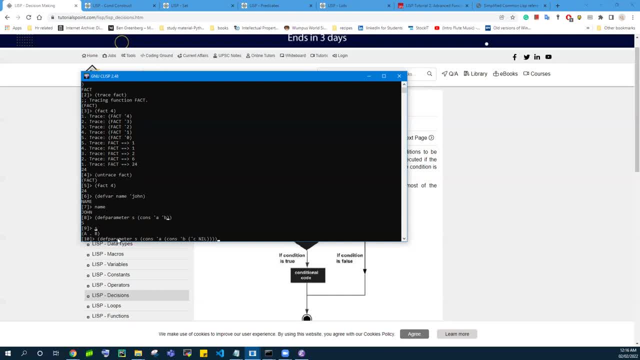 background, or it's also like the, it's like the ground, So this is a little bit of a tail thread in a linked list, like the one that points to nil. Let's see, We forgot to add the cons, So we have ABC. Now we have ABC. This is how. 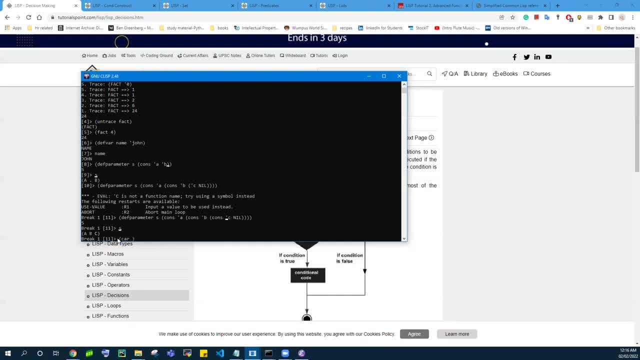 you add it. Let me show you how to char on it. So if you do a char on S, you get A. If you do a C, you get A cdr. on s, you will get everything after a. so, except for your first element, everything after that. 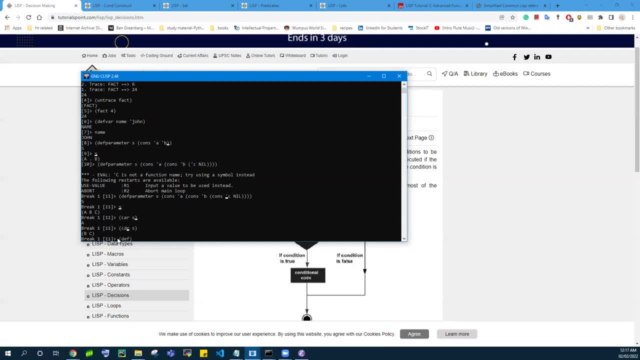 gets printed. so say you had a def parameter, a list of, say, a, c, d, e, f. i'm going to do a car on s, i get a. if i do a cdr, i should get b, c, d, e, f. awesome, how many times can you do a car or a cdr? you can nest them at multi levels. 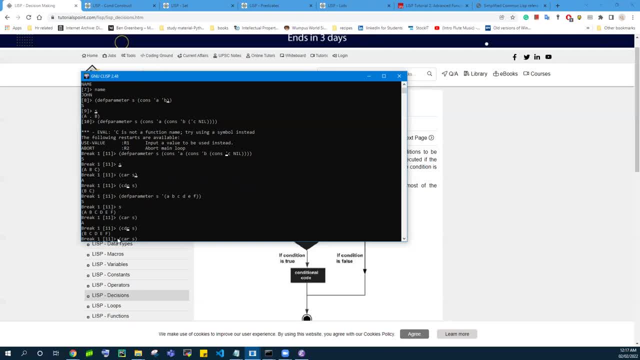 but a short way of doing it is say c a d? r. what will happen is first we'll take the c d? r, so it goes from right to left. so you'll first get a cdr and then it'll do a car on it, so you'll be 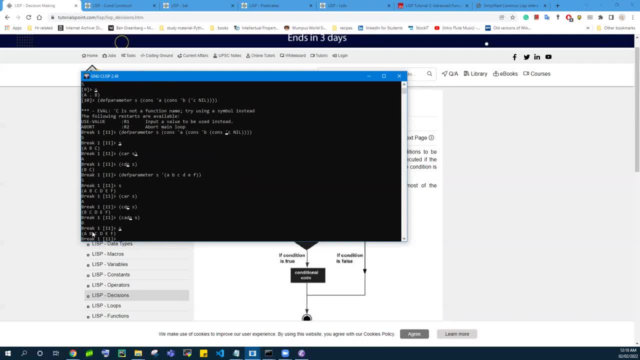 now, if you print s, you still have the original s, but this can be saved in a separate uh variable or a value and since it's a single atom, you can obviously do it with the def pair itself, with the def pair, although if you do it with the def parameter it shouldn't raise an. 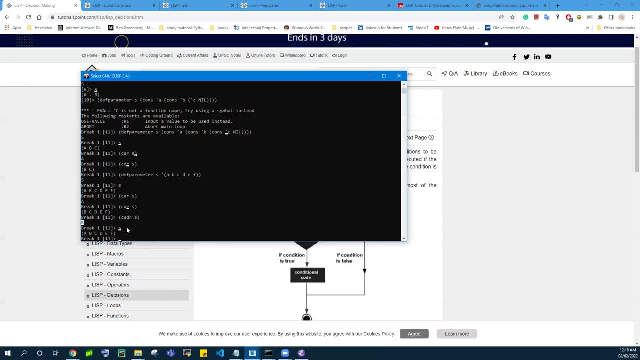 issue, uh, but if it's, if it's an item, you prefer using it with the def value and for lists with def parameter, we can nest these up to a certain level so you can have at most four of these inside. so you'll do a cdr and do a cdr, and do a cdr and then you do a car. so a cdr will be first b, c, d, e, f, another. 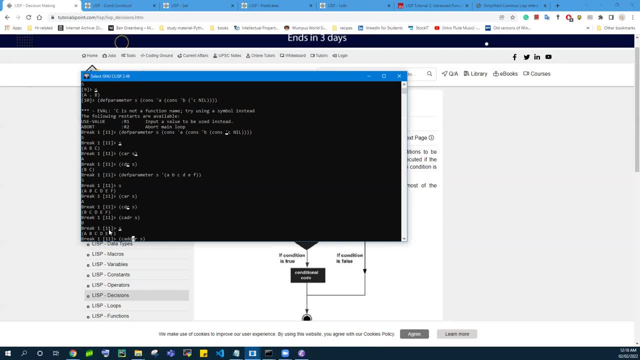 would be c, d e, f, another would be d e, f, and then you select your first one, which is d. sounds familiar, doesn't it? although if you nest it, uh, using the entire word, like you having a nest of, say uh, you can do it. the nest of, let's say, car and cdr and cdr, it's all it's going to. 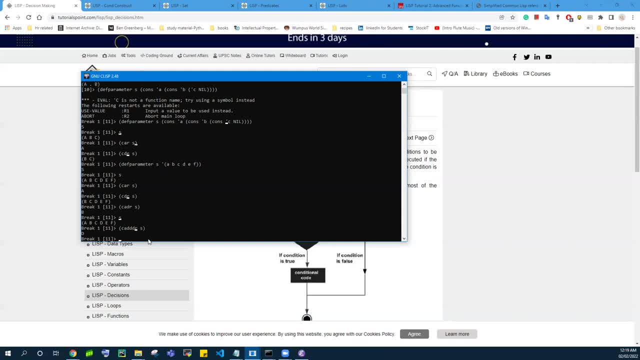 give you the same result. so, uh, you can do it whatever is comfortable with you, but but, as you see that you have a, c, a, d, d, d, r, there are four values out here. if you try to add even one more, it's going to break. let's, let's try that. we had a, d, e, f. 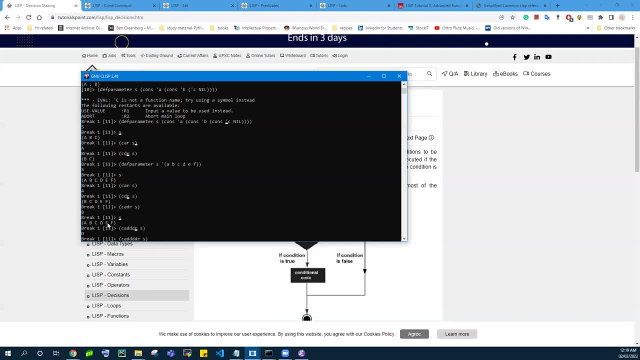 if we had one more d, you have gotten e, but this is what you get instead, because at most you can have only four uh points in in the nest at a time. so, yeah, that's something to look up to if we cut that out of there. uh, just remember how we can use car cdrs. 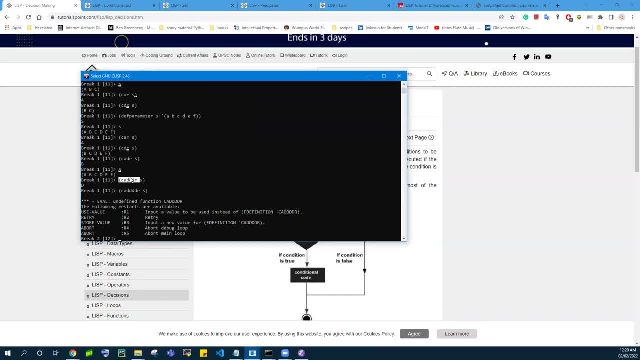 and how you can eliminate half of your list or eliminate a certain portion of the list so that you can get the rest of it. so maybe by the recursing you might want only half a list or only a second half of the list. do you know what to do now? talking about, uh, having the second half. 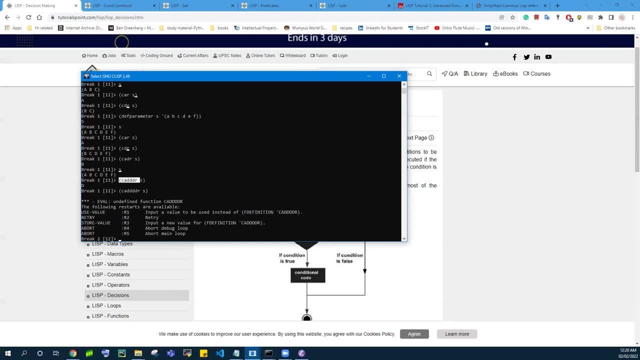 of it. let's go talk about the member function. so member is basically, or does this exist in that kind of a relation? so member will take will basically allow you to search for items inside your list and will return everything after a correct hit. so say, if it's found, then 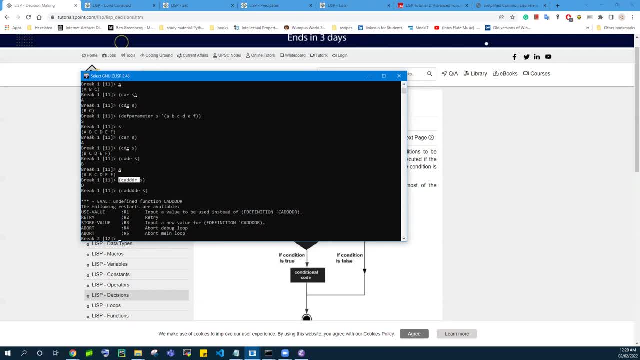 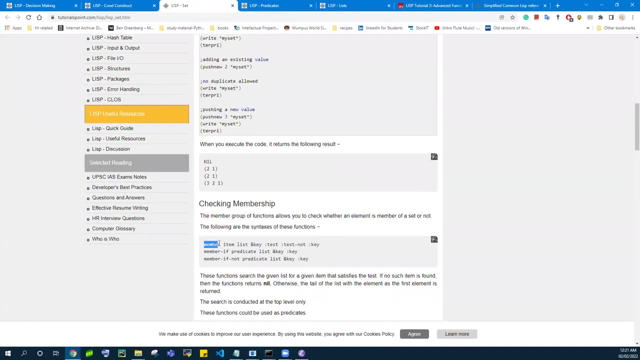 everything after your, after the value that you found. everything else gets printed onto it. let me show you how it works. it should be in sets: yep, so this is how a member looks like. you have other other ways of writing member also, but we will just stick to this one for now. so, member item. item is your atom or your? 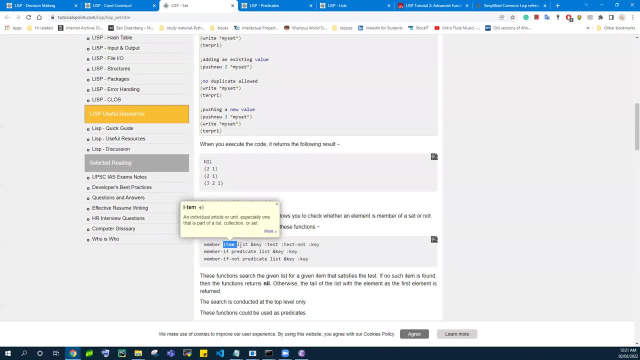 list or whatever you want to search for inside this list. so does this exist in this and you can use a test where you can modify whether you want an eq or an equal. we'll get to that later of how eq and equal is different. there is equal, there is. 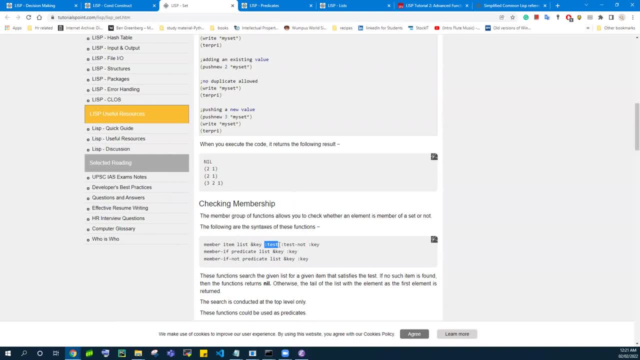 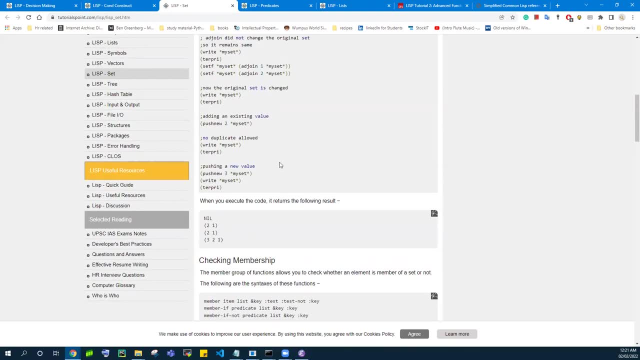 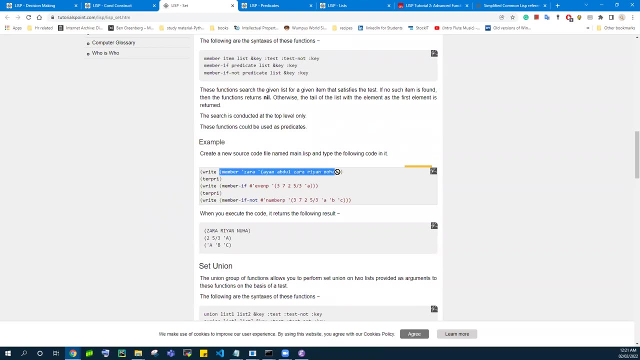 equal p, there is equal eq. there are a lot of them, but only some of them are of value to us. so yeah, let's take a look at a member. i'm just going to pick up a template example so that it's easy for me to copy. 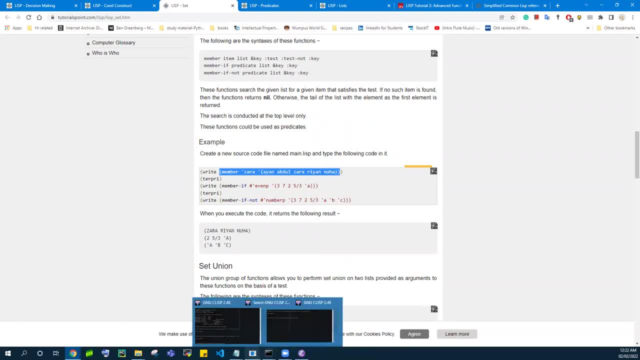 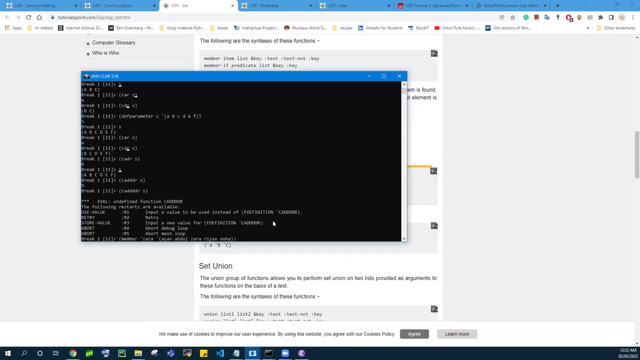 okay, let's go. okay, so is zara a member of this list? it is. so what do we get after? we find it, we get zara, we get ryan and nua. we get all three of them after the hit. so we can see that it first goes. it looks at ayan, looks at abdul, it looks at zara. it 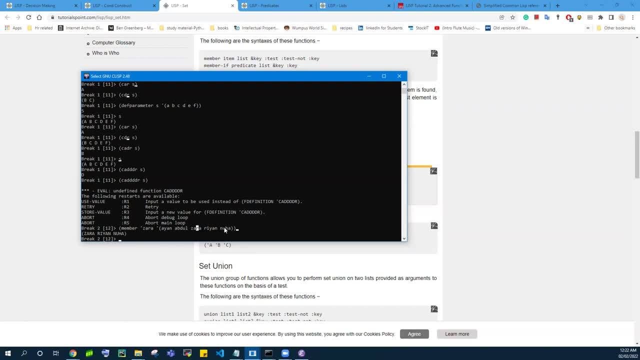 found zara, and then it just starts putting everything else. it's like it doesn't need to look anymore. it just returns everything after that. now, this sounds similar. this just looks like cdr, doesn't it? so if i had this list, if i do a cdr on it, 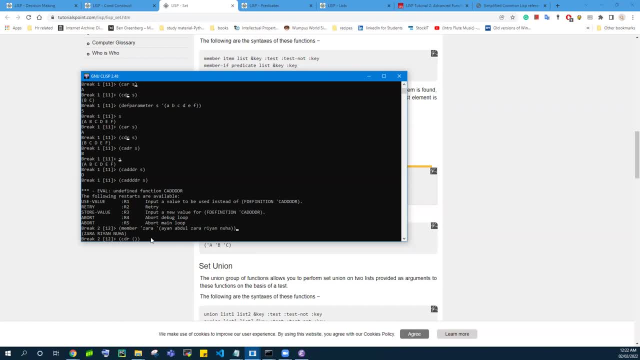 oh, okay, okay. So I wanted Sarah, So skip this, skip this. and that was yeah. So double CDR is what would what you would have achieved by using just member. So do we really need this? Maybe in certain cases yes, but if you're looking for, if you're searching for an element inside, 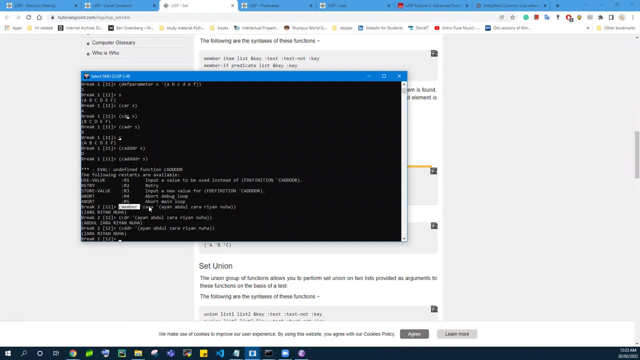 say, maybe you want to look if an element exists, or if you want to know if the element exists, and if it does, then you want everything after it, then you would use this, But if it doesn't, then you still want everything after it. then you're going to use CDRs or CADDR, depending. 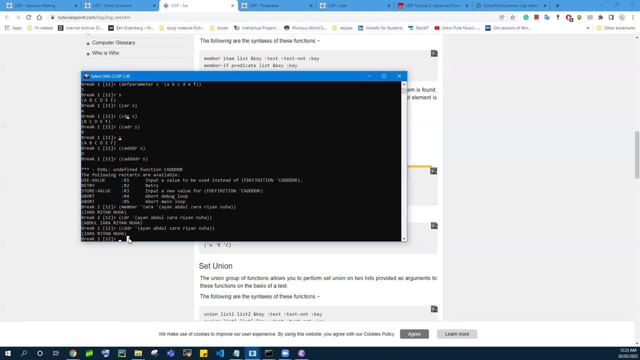 on. whatever your implementation is. Let me show you an example of where it doesn't exist. So let's say we have a full is full member of this? No, So it's going to return. So this is a case that you might have to handle. 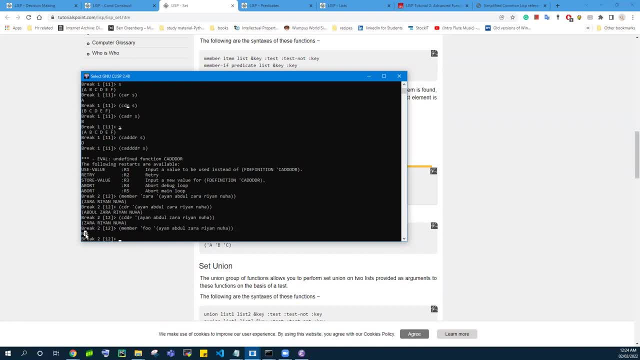 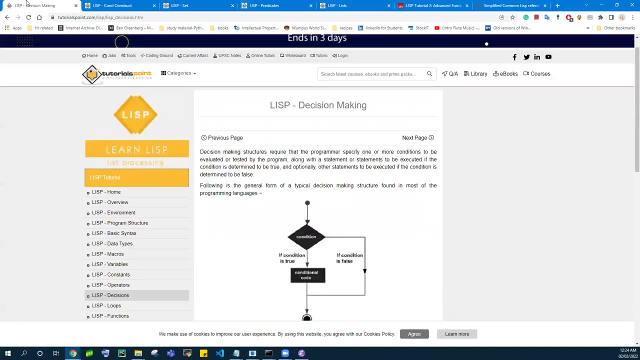 that if the element is not found, then it's going to return null. And since it's not found, maybe if you want to add it, you might want to add a condition and make sure it does add that. Talking about conditions, So we have a lot of decision-making that goes on in our programming. 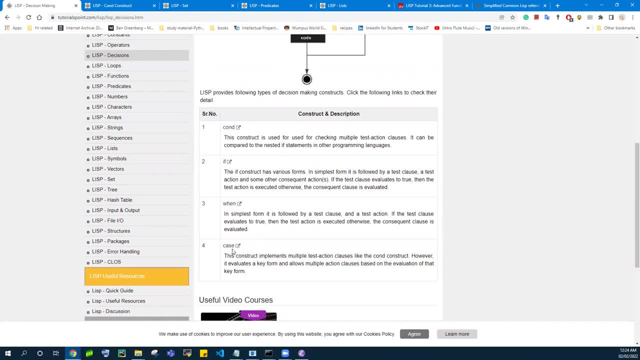 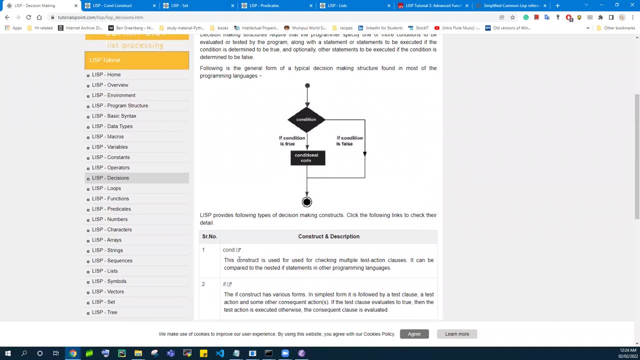 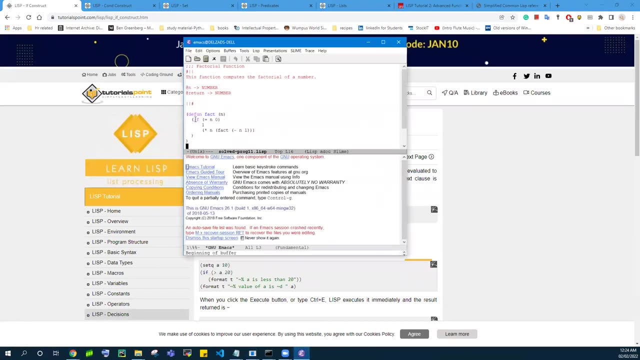 where you have a cond you have, if you have when you have case. I want to talk about if and cond because that is what we'll be using extensively. And if statement- you already used it before. You've also seen it for your this, the factorial program- that if this, 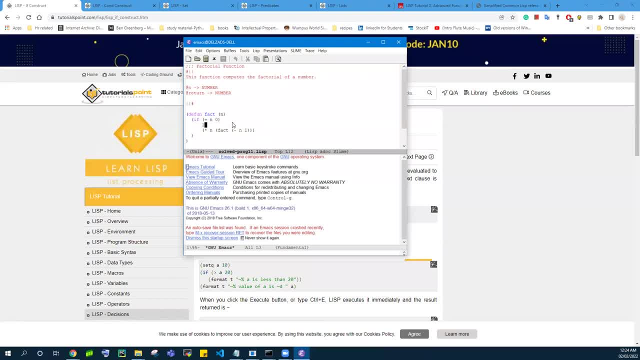 then this. So if you notice brackets in in a way that I can understand where the bracket starts and ends, So this is is the entire if condition, including the else condition. So if this, then return one else, return this. So what if you have too many conditions like, say, say you want to, you want to know if 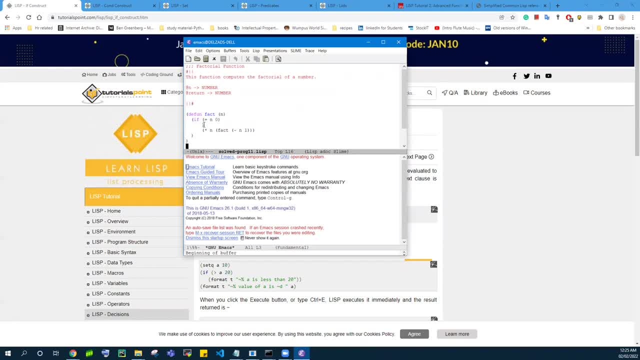 a person can uh drive. So say, certain places have a driving minimum age of 18.. Some have 21,, some have 24.. So like, if this, if country equal to this, then set it to 18, if country equal to this. 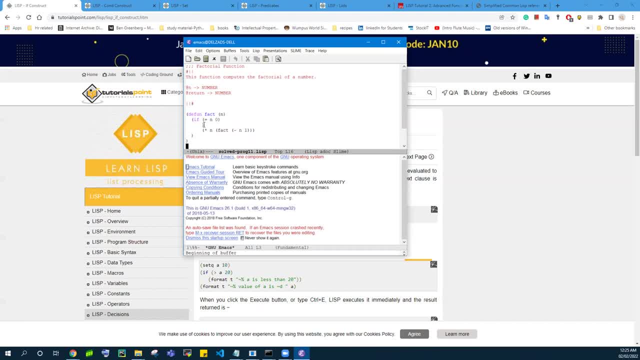 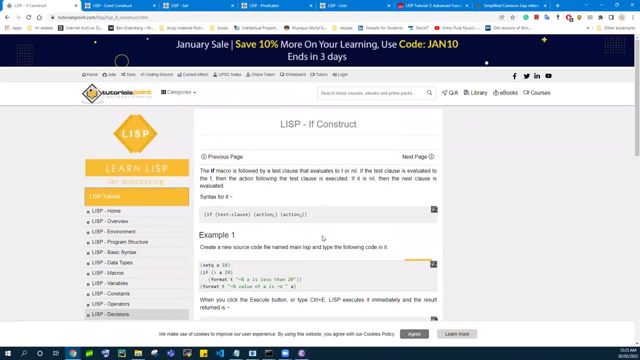 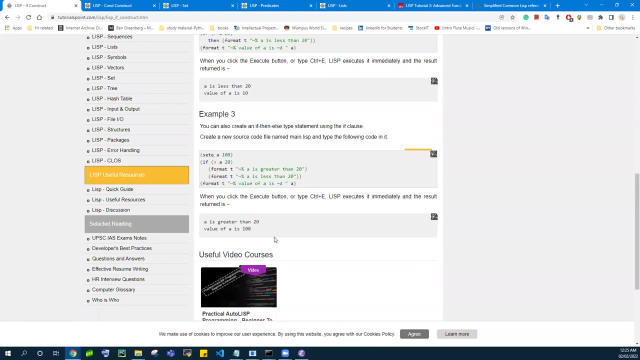 then set it to 21,. this then set it to this. So does it make sense of writing multiple if statements or going and getting confused in that, Of course, that there are multiple ways of writing it. Also, you don't have to necessarily only write an if, then or if else statement. you can, you. 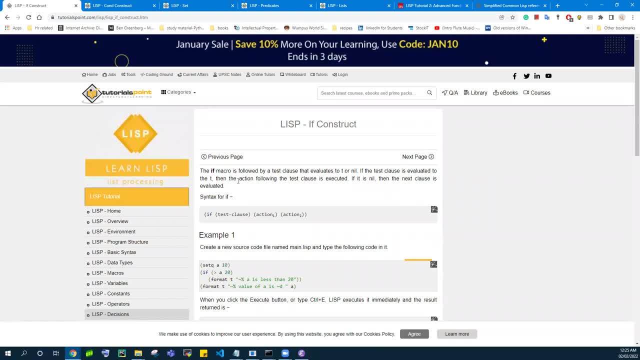 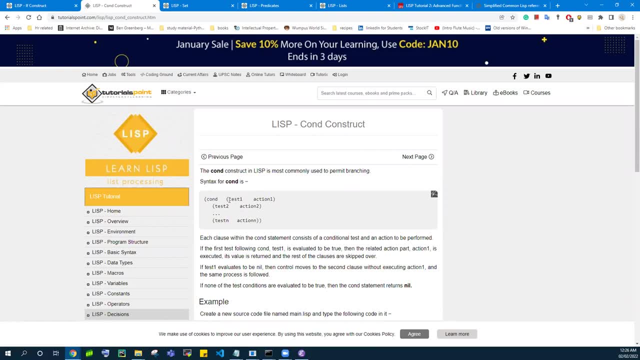 can nest them, but it gets a lot messier. That is why I suggest using COND C-O-N-D. It tests on multiple test cases, So it'll test on, say, uh, test one, then do this, test two, So test. 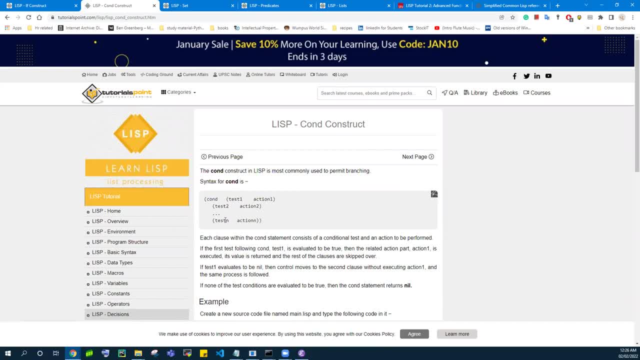 test one, two, three is basically just your conditions that you test, like your equality conditions or less than conditions, Or maybe if it's an atom, if it's a P, even if it's odd, then do this An action will. 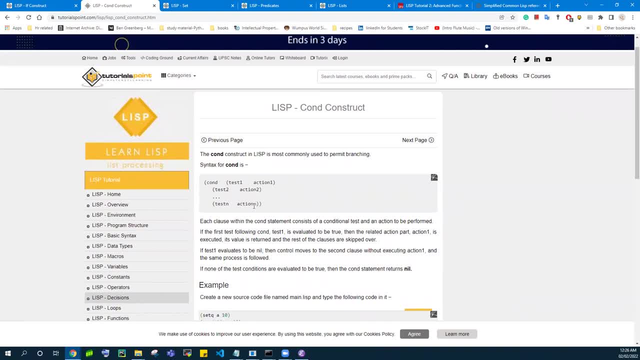 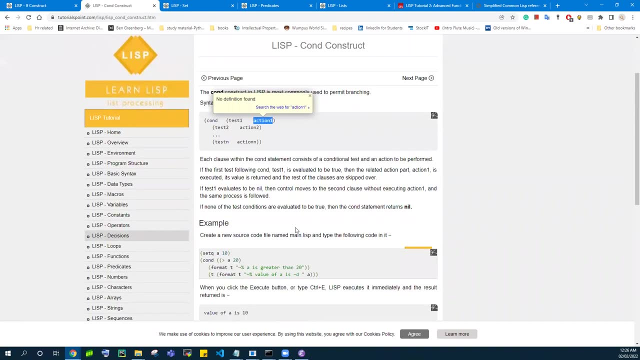 basically be what you want your uh if condition to perform. it could either be another say: if it's a recursion, you might want an action to be able to request something. If it's just the base case, you just want to return a value and not the rest of the function. So looking, at this out: here you're setting up a value. So if you want to return a value and not the rest of the function, So looking at this out, here you're setting up a value and not the rest of the function. So, looking at this out, here you're setting up a value and not the. 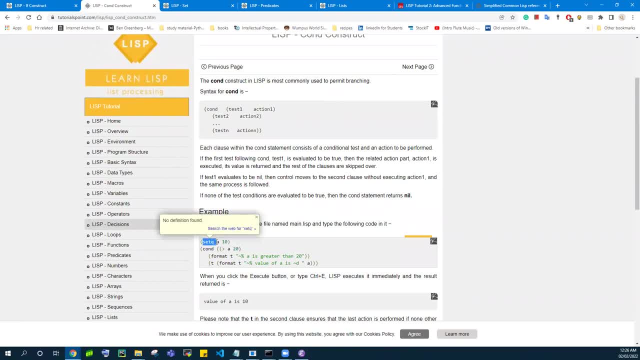 rest of the function. So, looking at this out, here you're setting up a value and not the rest of the function. So, looking at this out, here you're setting a as 10.. You can also use set queue to set have value. I used investment, but you can use set queue, You can use your. 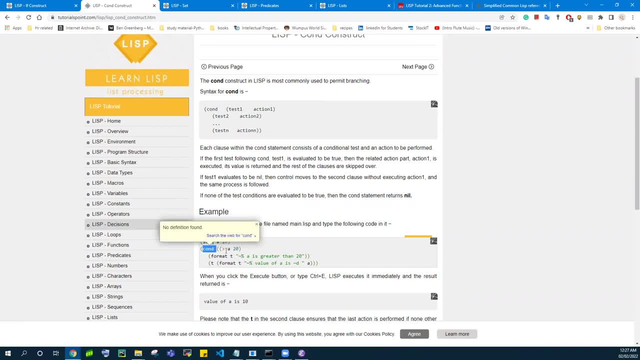 def parameter. You have CON A greater than 20.. Then do this Or do it's is A greater than 20? No case ten. So it's going to use this. So if you notice there is this T over here, uh, this T stands for true that variables. 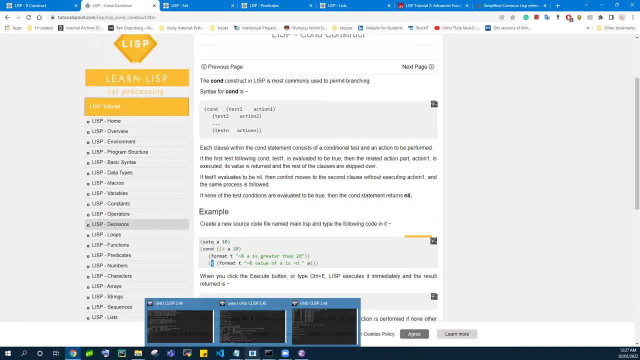 Yeah, all know about the true statement that we get if you search for, say, 10 more than five, you can sort on true, but out here this t acts more like a default value or like an else value that if any of these conditions inside are not true, then you can go ahead and execute. 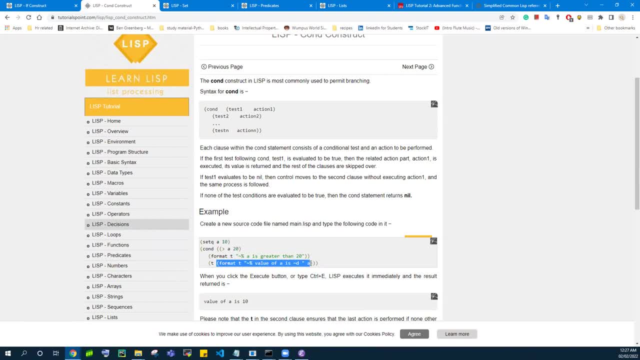 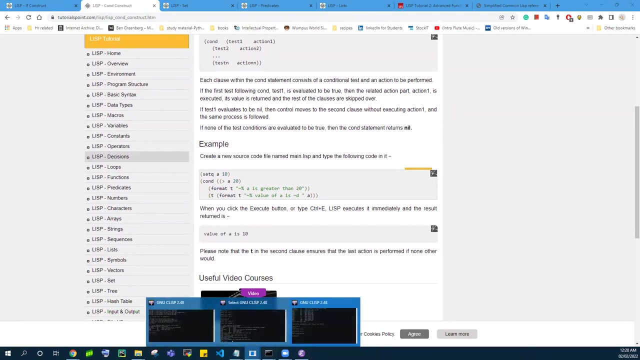 this more like a finally, but more of a quasi default finally else statement that will execute it irrespective of- sorry, not irrespective- but if any of the conditions above do not satisfy, then this one gets satisfied. so I wanted to show you an example of how you can use this, so I wrote- I found this. actually, I found this code online, where it will show: 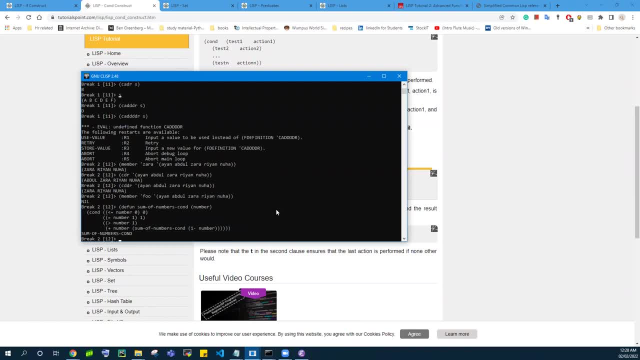 you a sum of numbers using the cond operation. so if a number is more than equal to zero, then return zero. if the number is equal to one, return one. if the number is greater than one, then add the number to the rest of it. so I didn't really like the way in the way, the way in which this code was formatted. 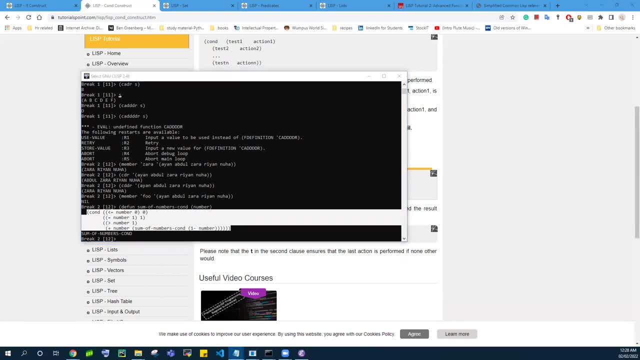 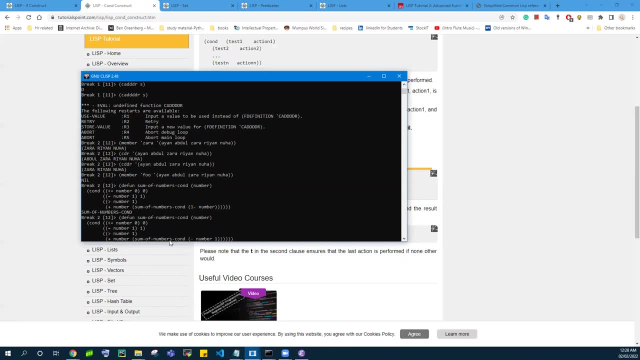 so I came up with this one that we're more familiar with. we've done something before, it's kind of the same, but here we have number minus one rather than having this shorthand subtraction. so if number plus the rest of the recursive function, number minus one. so 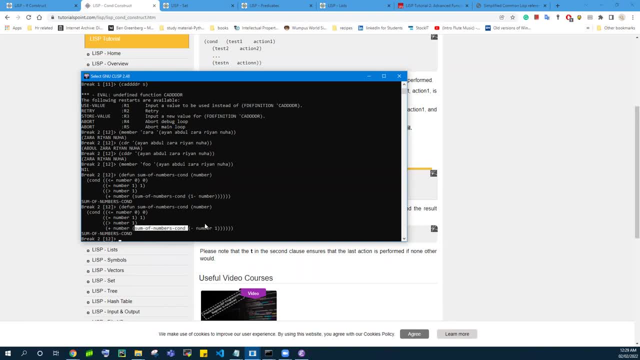 if, if you added four, it'll give you like three, two, one, and then then later on it's going to add one, two, three, four. but you want to simplify it further, you can just get rid of what is this? if it's greater than equal to zero, if it's equal to one, these two are base cases. but is this really necessary? this is where 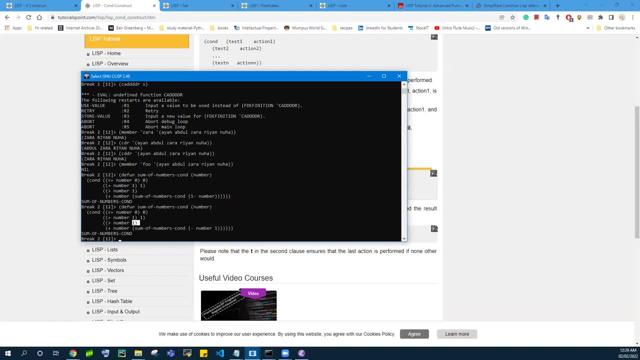 I would add the t to so say: you have this. all of these three functions do the same thing, but they're just written a different way. sum of numbers- zero, one greater than one, then do this. zero one greater than one, then do this or this. so you should, if you, if you take a look at this. so this is my default t, if. 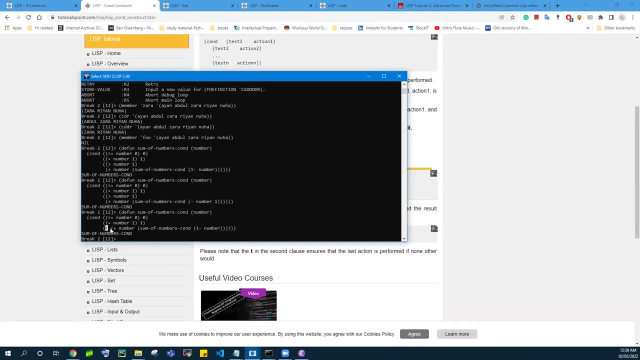 it's not zero, if it's not one, then by default this is going to go ahead and let me trace it and show you- and this is why I keep pestering you all about the trace thing, because it it really does help understand uh, how, uh how you can use it. so let's say I want the sum of numbers, say three. 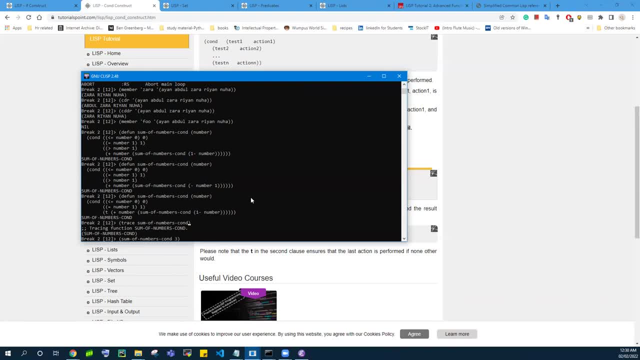 so, intuitively thinking, three plus two plus one, it's going to give you six. but let's see how it breaks down and you can see it on the screen. it's going to go from number three. the original number goes in. is this true? no, is this no? so by default, number plus power, blah, this goes on. you get two. 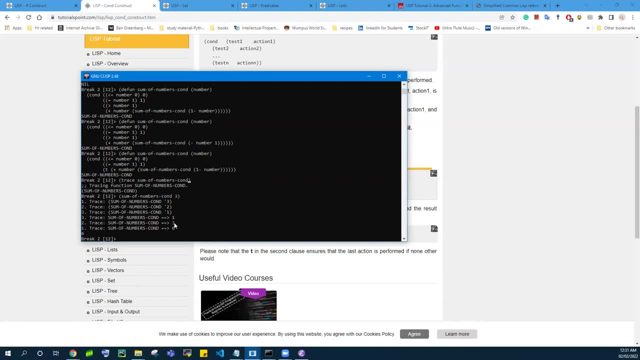 then you go to one and then starts the addition part of it. so one, three, two, so two plus one becomes three, three plus three becomes six, and that's how you get the six back. okay, so please get get used to call, start using code, of course, if you're not going to penalize you, if you're going to use if, but 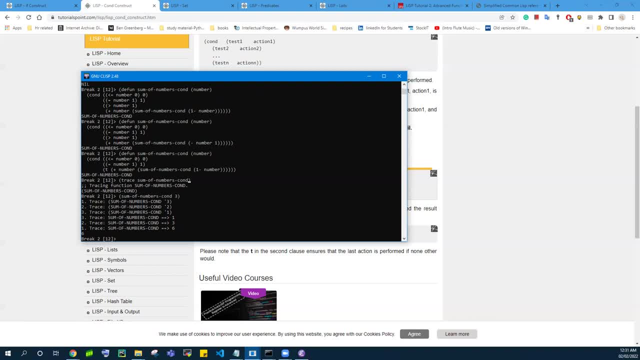 uh, you're just going to make it worse for y'all. um, coming back to the eq: equal and equal. so let me show you an example of what I mean by eq, how, how eq and equals are different. so three is three, that should be true. three four should be false. 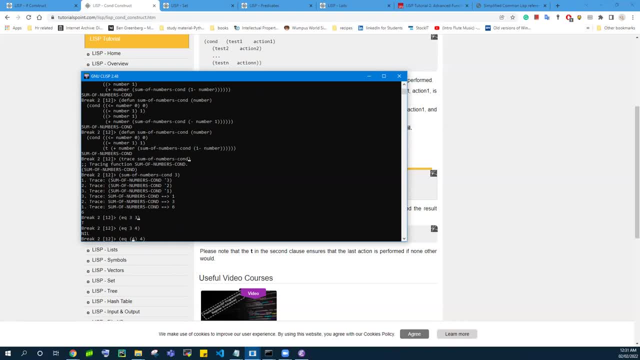 now, if I do this, some of you might be like, hey, this look exactly the same. this is just for an ad, a list of four and list of four. so it should be true, right? nope, this gets stored in different um address point. this gets stored in a different address point. 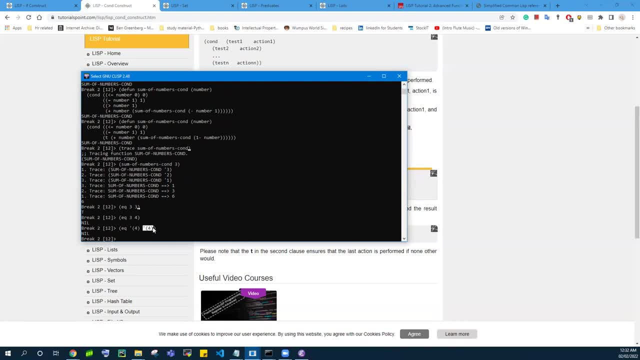 that is why they're not technically equal. I mean, they are equal, but the eq does not satisfy it. but if you look at just the value, just the value is, it is basically like: so, if you use javascript before you know how, there is a strict check, strict equals check, and there's a regular check and the regular. 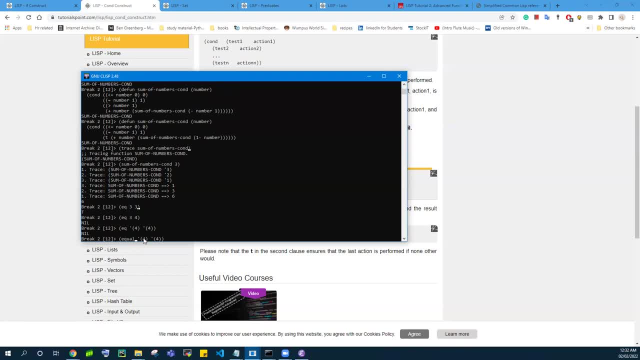 check, everything that matches the values gets gets true. it's precisely what happens here. with equal Treat, everything gets by default selected as everything is searched by value. but let's say you have something like this: oops, isn't this the same value as this, but the data type is different. 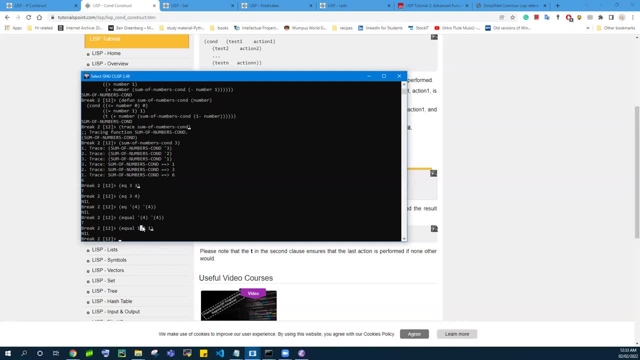 right. so this is a float. I don't know what it's called in this, but I mean it's a decimal value. we're going to say it'sget artirστicc and this is a number. so how do you go across about that? there is another one known as equal. 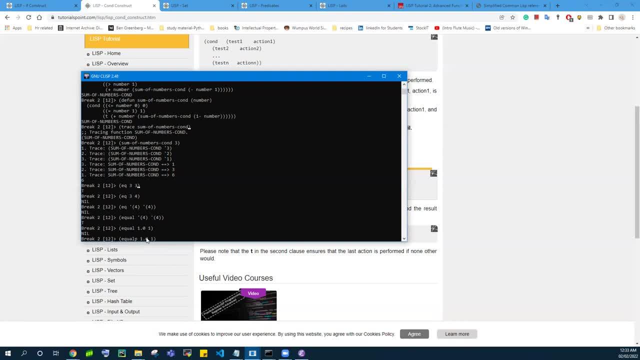 p, which kind of overlooks even the data types. these are just nasty ways of making lives more complicated, but they have their own purpose for sure. equal checks for value, but it does not look for data types. equal p just is just true for as long as it the value matches eq. it's a little more stubborn about things, so you might want to just. 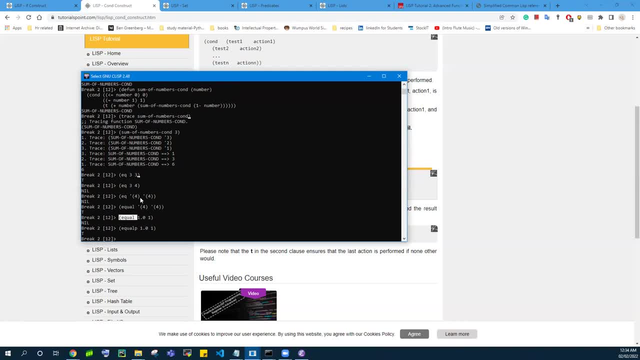 play around, practice, figure out what's up. another thing i wanted to let you all know is what about null and nil? are these two guys different? you are the same. from from the look of it, it is the same and that is exactly what it is. so a null, nil. 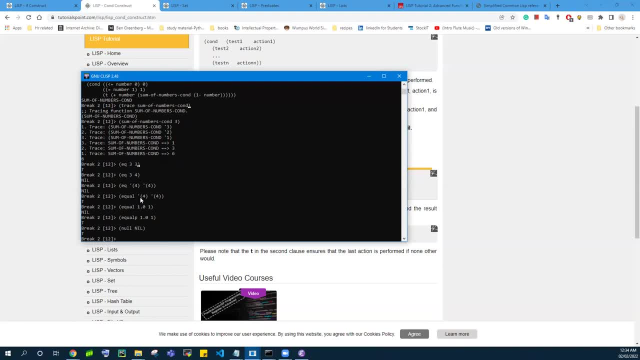 should return true because you're checking if nil is null. remember how it goes. nil is none, it's, it's in the prefix order, so yeah, so you're going to be using this a lot in this homework. you're going to be using member a lot. you're going to use number, you're going to use symbol, you're. 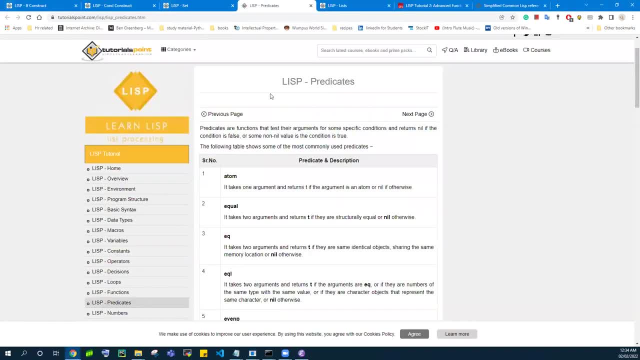 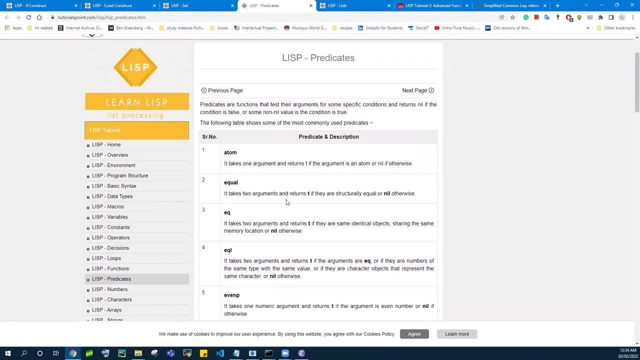 going to use atom. let's talk about predicates of the atom, and i just spoke about atom and everything. so let's see what exactly is an atom. an atom is basically a single value and a single, any single values. it could be maybe a number, it could be a symbol, it could be maybe any alphabet- a, b, c, d. it could be a. 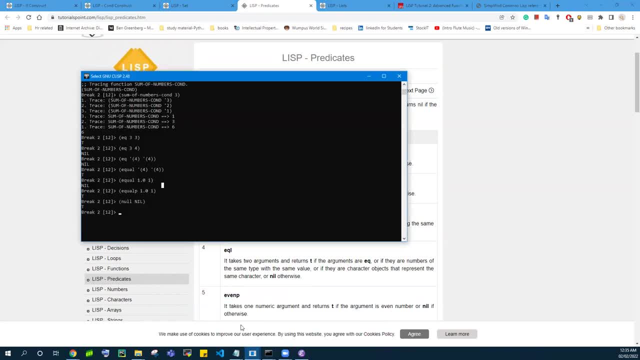 string anything at all. so how does it go about? atom a should be true, atom one should be true. atom, say john should be true, atom nil should be true. but if i do atom, so an ad, a list, can never be an atom right, because it's not a single valued item, a list, even even though a list, even though a list. 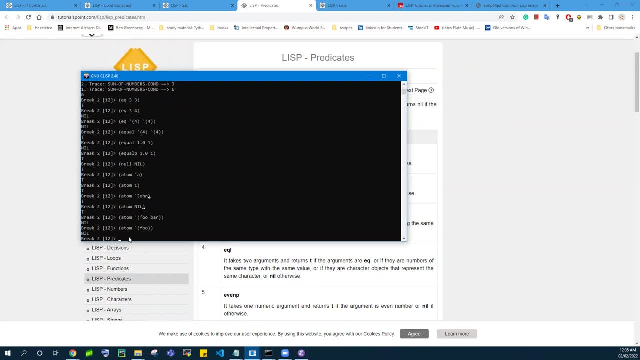 is a single valued list, it is still not an atom, because any it it could have, it could increase, it could become uh more than an atom, right? so this is is a check for uh, whether you, if, whether you have just a single value, you have a list. and if you have a list, then what are you going to do ahead with it? 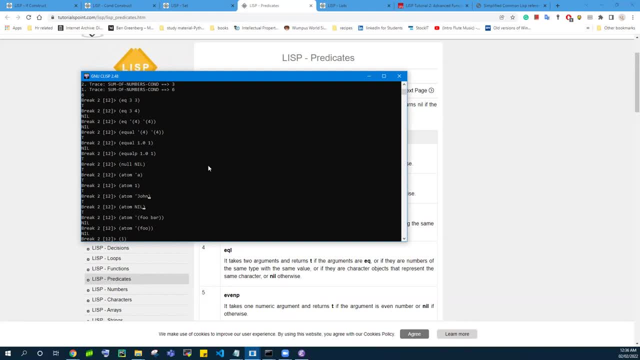 uh, now, what is this one? this is just a number, right, so would you have to check if, if it's a number or not, so is instance of integer or is instance of alpha? uh, if people have done python, you'll know like is alpha will basically turn if it's an alphabet or not. is num will tell you if. 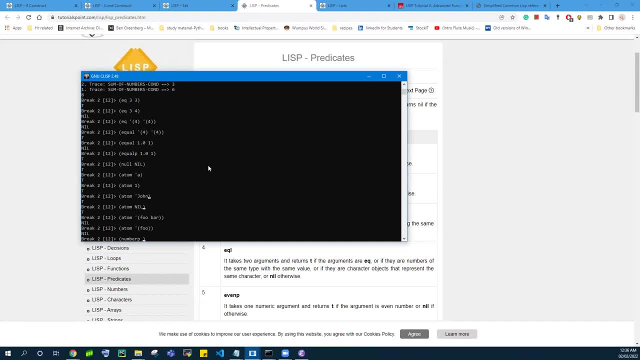 it's a number or not. so, similarly, we have number p, which will tell you for number: if, if, if, if an atom is a number or not. but if i do, if i do it as a, it's not a number, similarly. so you don't have a check that i know of. for 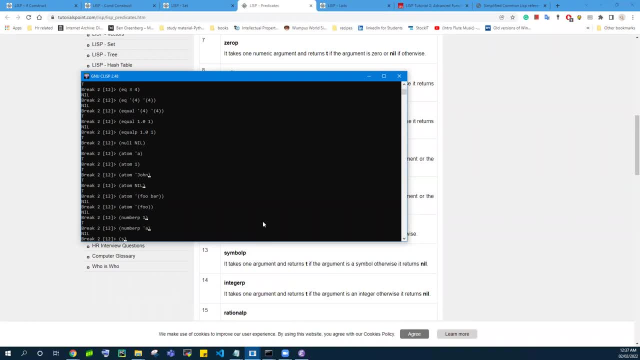 uh, oh, you do have a symbol p also. okay, so if, if you want to check for symbol, you could just do: is one a symbol? no, but is a symbol yes. yeah, so it just makes it like more easier. but do you really need that? you could have just done a not. 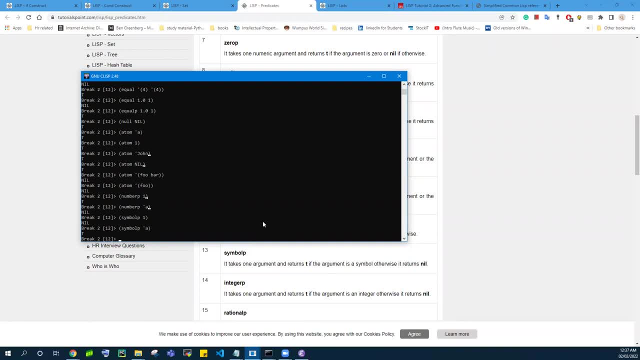 or a number p, and you would still get the same thing right. so kind of useless. but i mean it's simpler this way if it makes it easy for you also. yeah, uh, yeah. so just look up for number p, if it's a number or not, if it's an alphabet or not, and atom, for if it's a list or not, might strike. 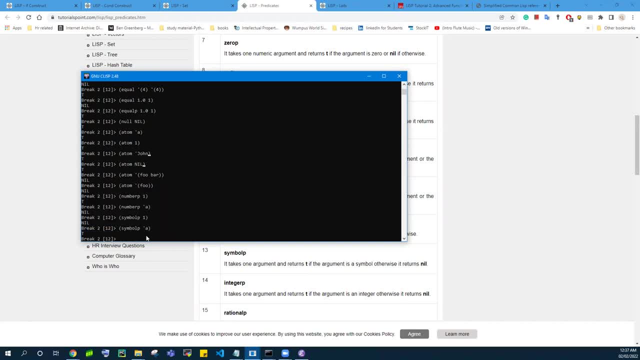 something. maybe, maybe not take a look odd be. um, just while we're at this topic, i'll just take a. i'll just make you all go through this. so if, if you have an odd number, it's going to turn, true if you have an even number. 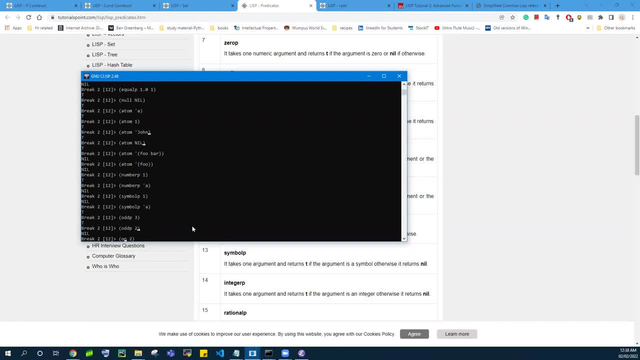 put it on false. similarly, even p will also do the same thing again. so it doesn't make sense, honestly. uh, i think, knowing two separate things, you could have just done a, not on one of them, to make a true, false and then recurs on it. but yeah, whatever, whatever is comfortable. 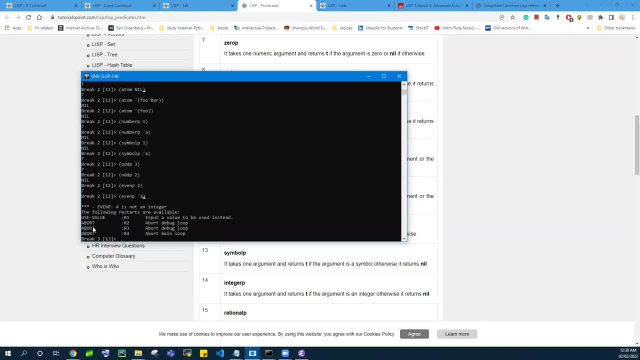 what if you just add something random, very stupid, then it's just going to be like it's not an integer right it. so just be careful of that. if, if you're using on p or even p, uh, you want to have numbers itself, you can't just add something like a list or 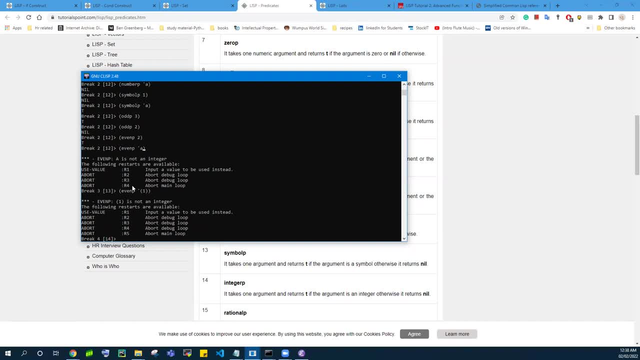 something random. it has to be integer atom, integer atom. yeah, okay, so you've gone over this. you've gone over equals. anything else that i need to check for the homework? yeah, okay, so i think we're good to go. uh, you could just take a look at it, i'll just make. 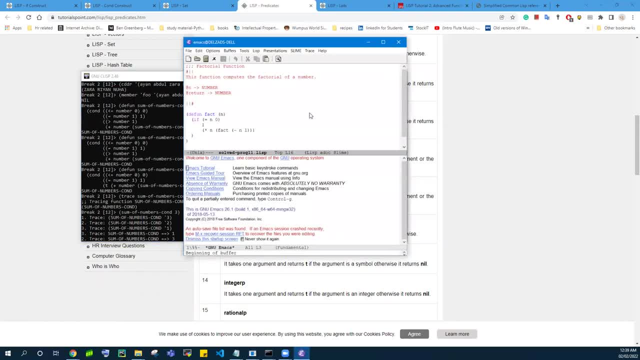 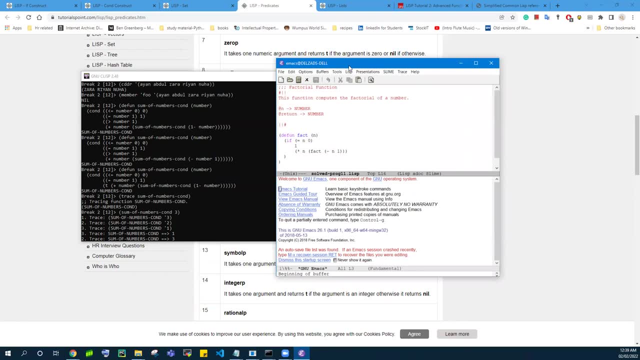 you go through recursion once more, once using if and once using on um. feel free to use whichever you want. please preferably use, and it'll make your and our lives easy for debugging. and if you're using it, please, please, please, make sure you use it: indent your brackets correctly, because otherwise it's going to be a nightmare. 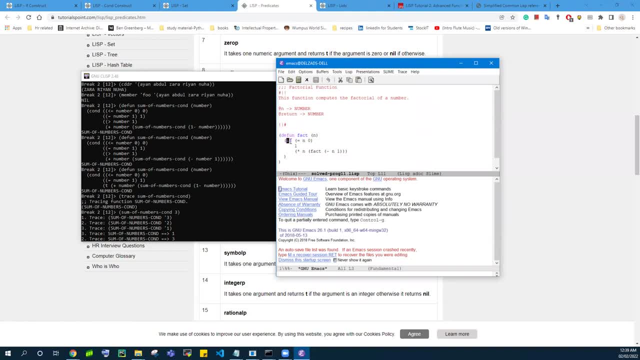 So if you're using, if you're going to have an if condition, you're going to have a base case and everything in your else will be your tail recursion where you'll be recursing on it. so you'll remove the first element and then you check on the rest of it. 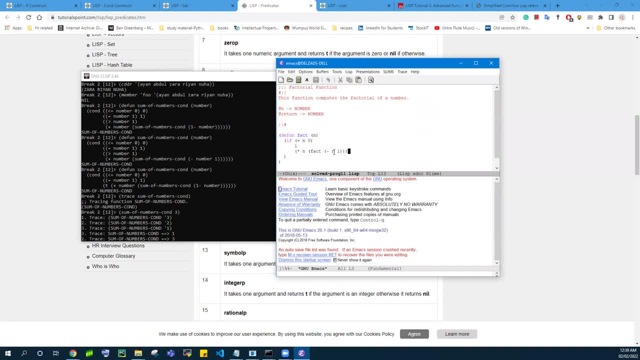 Remember, you could use cad, you can use cdr, you can use member, you can use whatever is feasible, whatever is applicable and whatever makes sense to that question per se. Don't kind of make a rookie mistake where you think that hey, I can use member wherever I want. 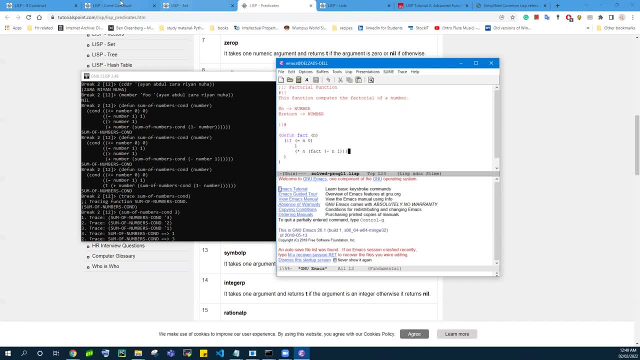 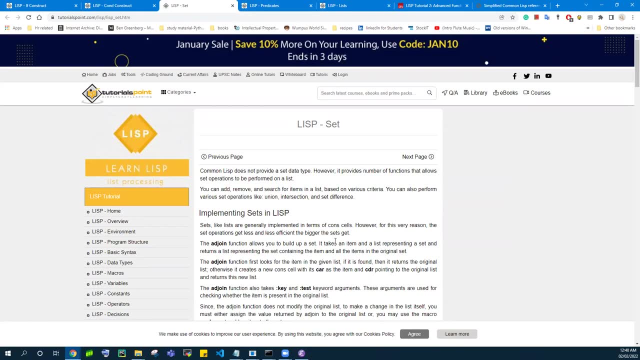 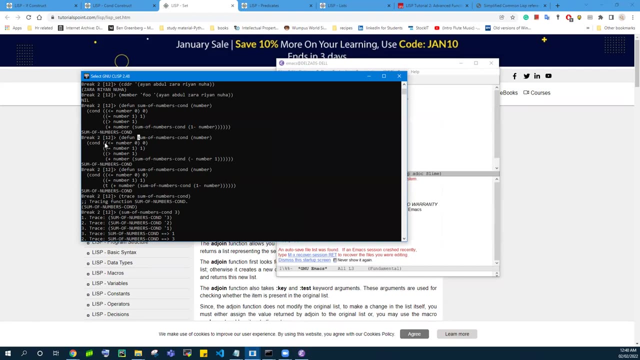 member has its own limitations. do look it up. it's right here. tonic point, google all the way. it's always helpful. When it comes to cond, as I mentioned, you have one bracket here, one bracket here and sorry, it's in the end. oh no, it was like I was trying to force that. yeah, so this is what can. 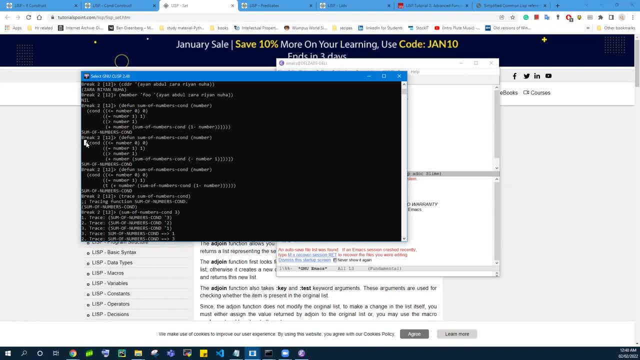 happen. so if you don't have it intended correctly, you're just going to be like: wait, is this closed? no, is this closed? no. so just be careful about that. this ends this. this ends the con inside the con. you like if you'll be adding everything inside the con bracket itself and then you'll have like 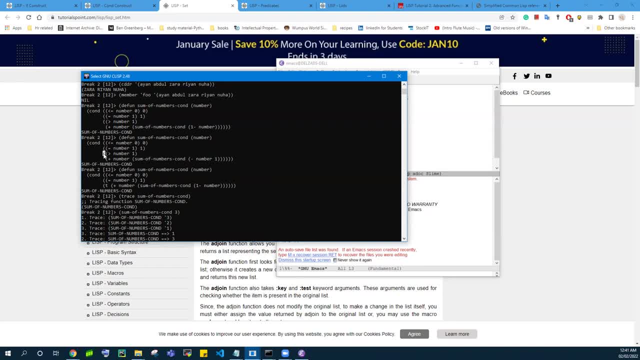 case one, case two, case three and the what happens in case three. So, as I mentioned last time, you can use your action does not necessarily have to be just an atom. the action for this condition is this entire thing. This is the action. this is the case one. you return zero. if this is true, 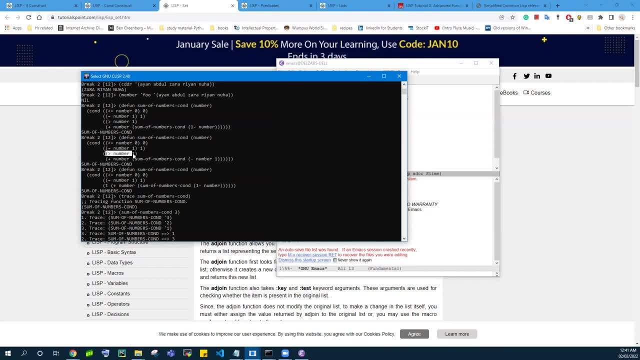 you return one if this is true. and if this is true, then you do this entire thing. So your action can also be your tail recursion and you could always shorten it with the t. You could definitely look up for more tutorials. you can look up the tutorials point where I have. 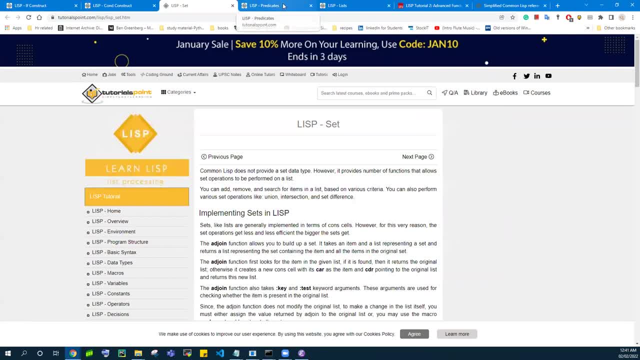 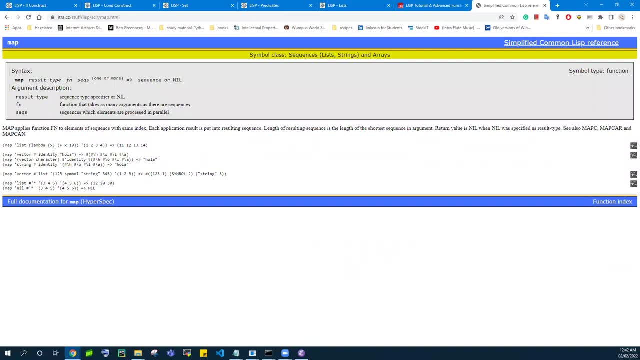 added these few. if there is con, there is set. there's predicates lists. Oh yeah, we can let me show you how that works. I'm not sure how useful this would be, but it's always good to know, since you've started it. 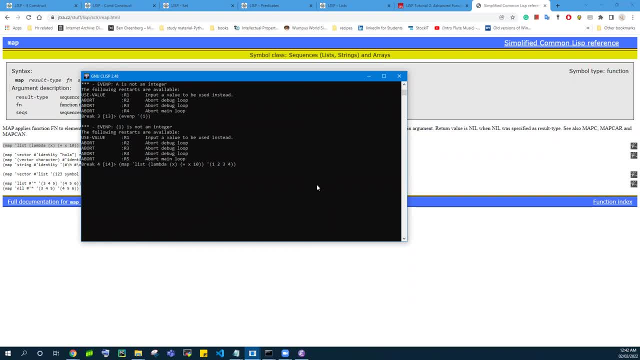 So you've used any other functional programming language before You know what a map does. You will be mapping over this entire list and you'll perform this function on it. So this is like an anonymous function if you're aware of it. So an anonymous function is a function where you don't really have the 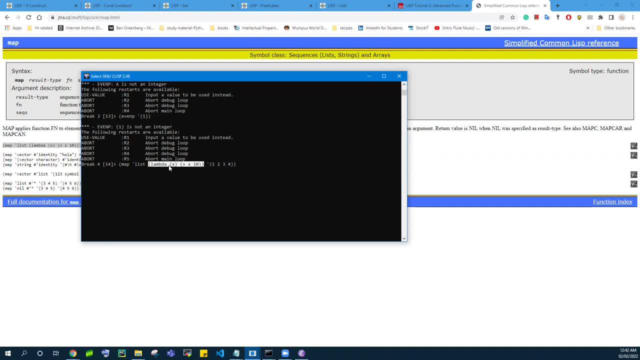 function saved somewhere or like have the name or something of it, but it comes as a part of implementation itself. it just comes as a part of the implementation. So it's just like you can just get implemented on this on the fly. It's just done on the spot. 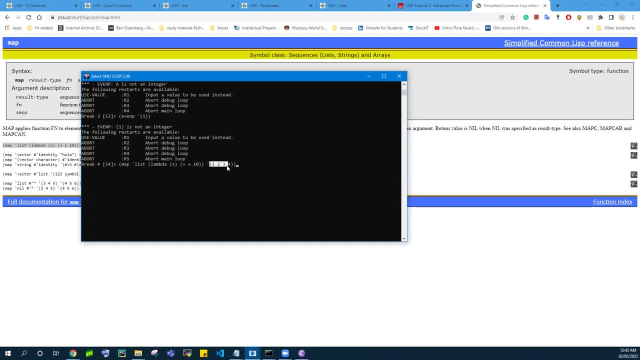 So what are we doing out here? We have a list- one, two, three, four- and we're passing this anonymous function to it, where we pass x onto this. I mean, we pass the value of x onto this and we're going to map each value of x and add it to 10.. This would give us 11,, 12,, 13,, 14.. 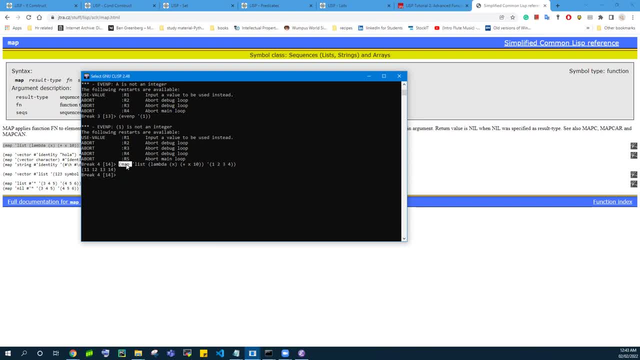 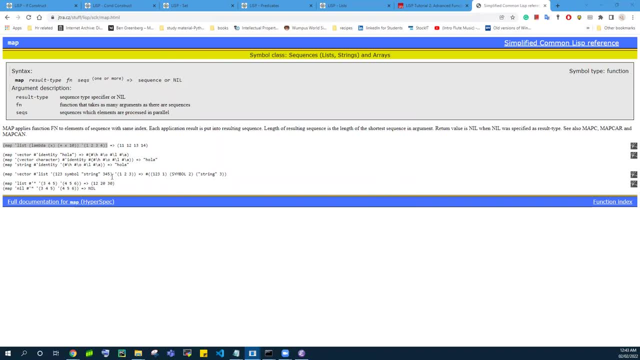 So this is how you can use map. You could play around with it a little more. You could, as you see out here. I'll attach this to the link. I mean, I'll attach this to the description. You can see how you can use different. you can use map in a different way. 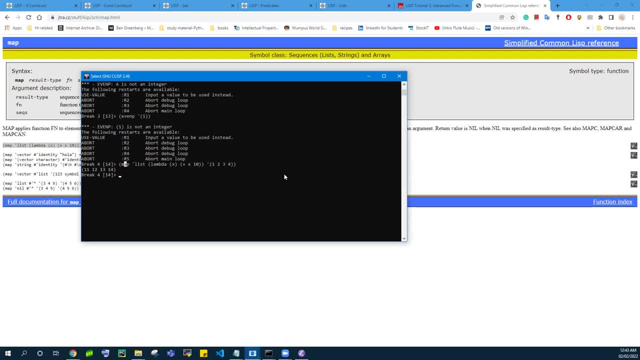 I also want to introduce you all to reverse. Say, I have a list def s. I have one, two, three, four, five and s. Now I'm going to reverse this 500 to 1.. What if s was letters E-D-C-V-A? So yeah, it works in that. What if p is a mixture of integers and? 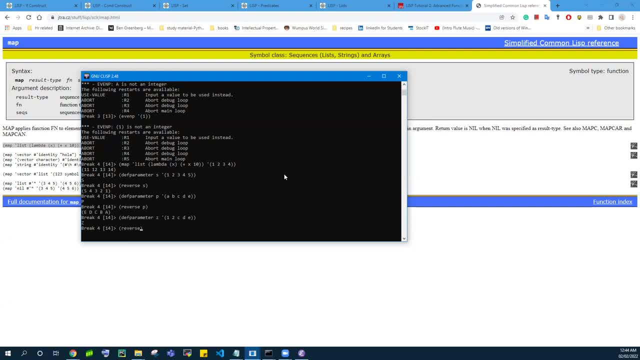 and letter symbols. So this is going to act funny because you will be having a mixture of, uh, letters and numbers, but they will don't be any exact way of determining whether this is greater or not. Like if you go, if you try to remove, like some ask i value or something. 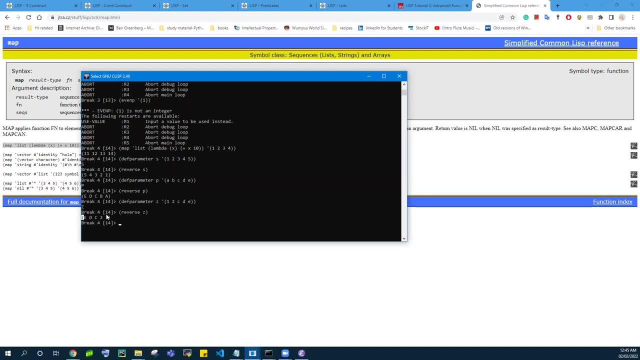 it's not going to be in this order, but it's just that it's going to follow whatever order you put it in, It's going to follow it in that way. So let me try putting it, and we put two here, Maybe I'll put a here and then I do reverse E-D-2-a-1.. So you see, it's not following any. 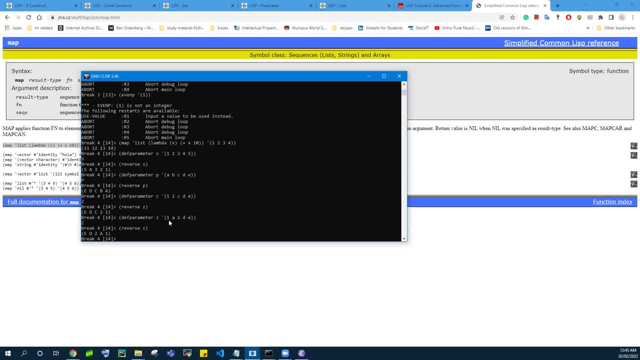 specific pattern is just taking the entire list and blindly just reversing it. uh see if this is helpful, see if this is useful. look up different functions, look up different, uh, ways of using it. obviously, uh see if there is a way of putting an element inside a list. that's definitely not.